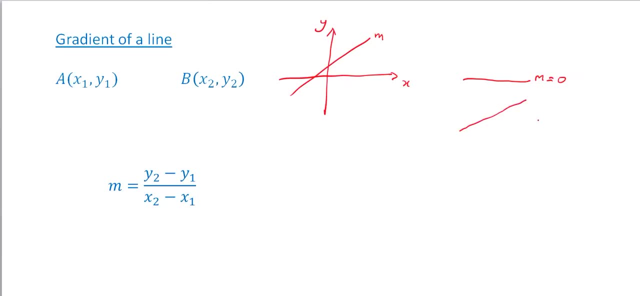 If we have a line that is sloping upwards, then the gradient is positive. If we have a line that is sloping this way, m is negative, And if we have a vertical line, m is equal to infinity, right? So if we have a line, let's say like this: and gradient m is equal to 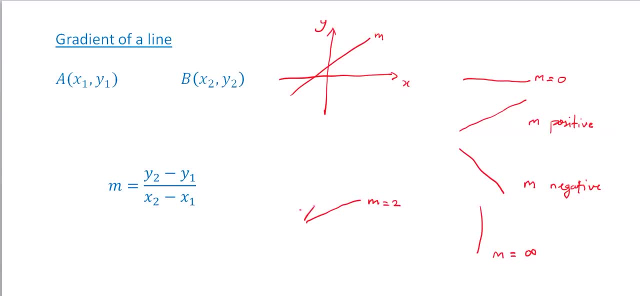 two. And then we have another line which is even steeper. then m should be larger. So m could be something like three, right? So there is a formula to find the gradient of a straight line, given or provided that we have two points on the line, right. 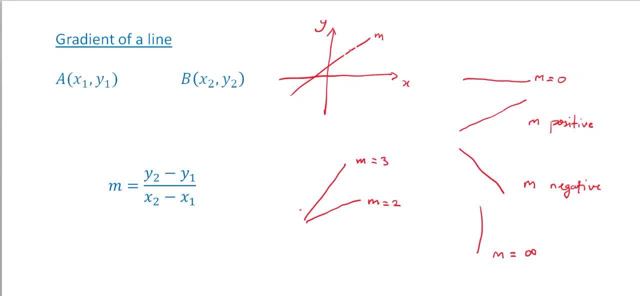 So let's say we have a point, point a, and another point which is b, And the coordinates of a coordinates of a is x1, y1.. And the coordinates of b is x2, y2. Then the gradient is given by y2 minus y1 over x2 minus x1. 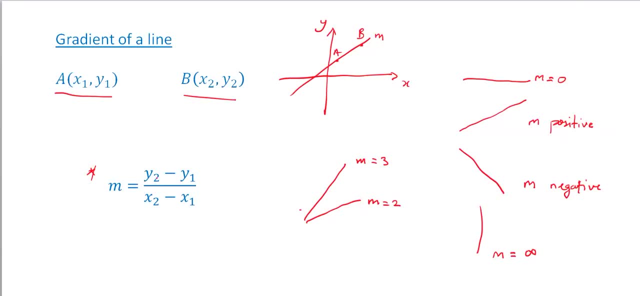 I need to remember this formula And just remember it's the difference of the y-coordinates on top divided by the difference of the x-coordinates at the bottom. So let's say, suppose a was 2,, 6, and b was, let's say, 4,, 12, right? 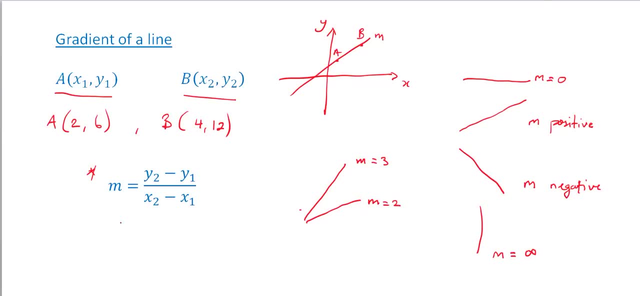 And we wanted to find the gradient of the line a b. Then if we use the formula, m is equal to right now. you see, at this point here, whenever you have the two coordinates you need to make sure you know in your head. 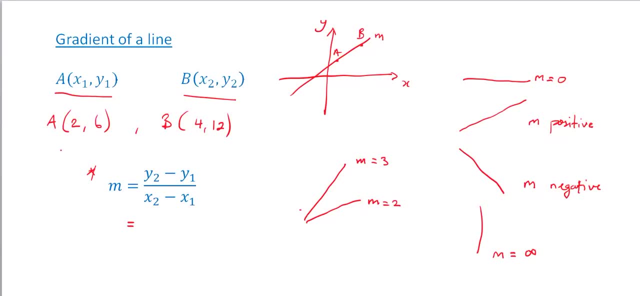 which one is x1,, which one is y1,, which one is x2, and which one is y2.. So we can choose any one of the points and call it x1 or x2.. So let's say, let's say I use a. 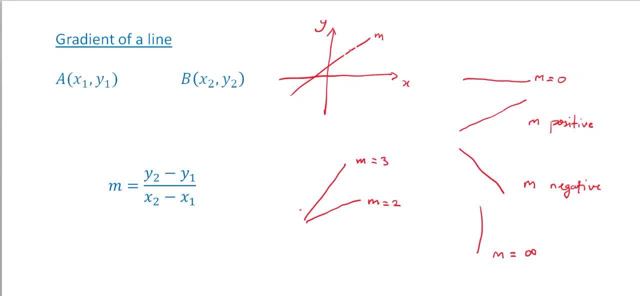 So let's say we have a point, point a, and another point which is b, And the coordinates of a coordinates of a is x1, y1.. And the coordinates of b is x2, y2. Then the gradient is given by y2 minus y1 over x2 minus x1. 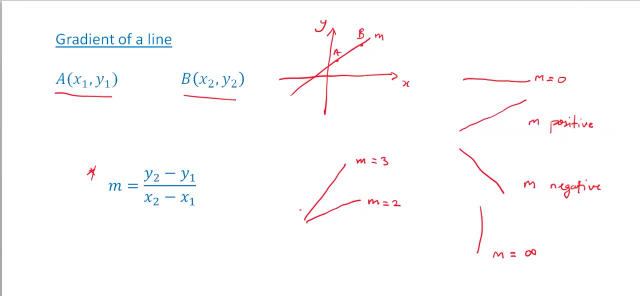 I need to remember this formula And just remember it's the difference of the y-coordinates on top divided by the difference of the x-coordinates at the bottom. So let's say, suppose a was 2,, 6, and b was, let's say, 4,, 12, right? 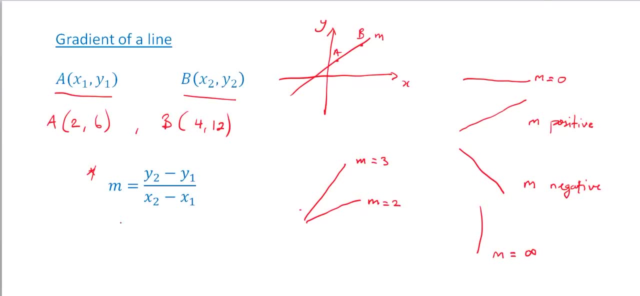 And we wanted to find the gradient of the line a b. Then if we use the formula, m is equal to right now. you see, at this point here, whenever you have the two coordinates you need to make sure you know in your head. 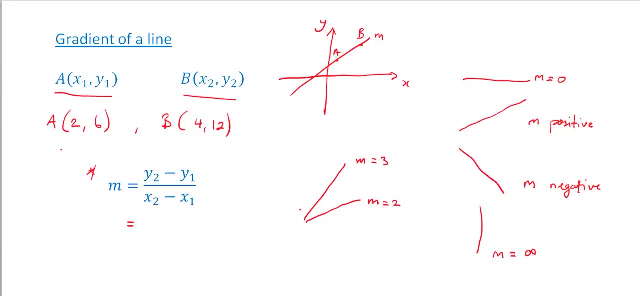 which one is x1,, which one is y1,, which one is x2, and which one is y2.. So we can choose any one of the points and call it x1 or x2.. So let's say, let's say I use a. 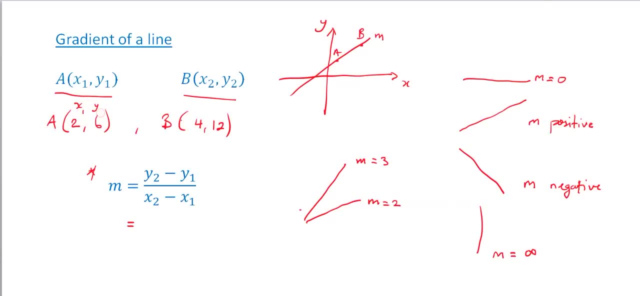 let's call this x1, I call this y1.. If I need to call this x2, I call this y2, right? So what you can do when you have the coordinates, just put a quick label on top of the coordinates so you don't get confused. 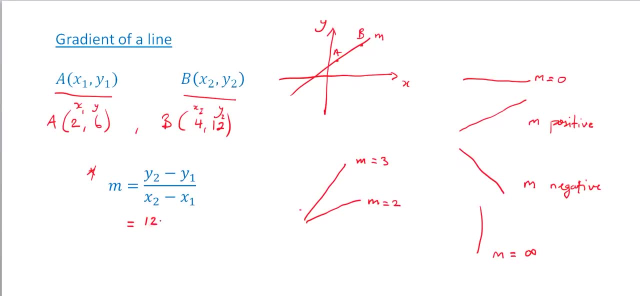 So it's y2 minus y1, so it'll be 12 minus 6 divided by 4 minus 2, and that gives me 6 over 2, which is equal to 3.. So the gradient of the line a b will be equal to 3, right. 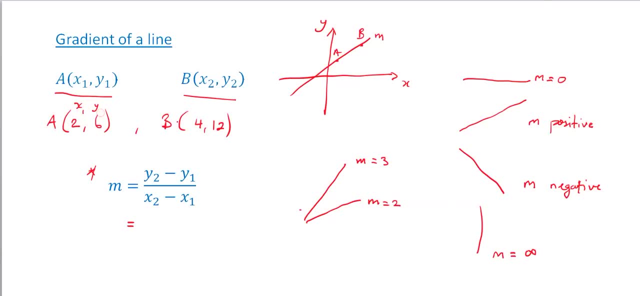 let's call this x1,, I call this y1,. therefore, I need to call this x2, and I call this y2, right? So what you can do when you have the coordinates: just put a quick label on top of the coordinates so you don't get confused. 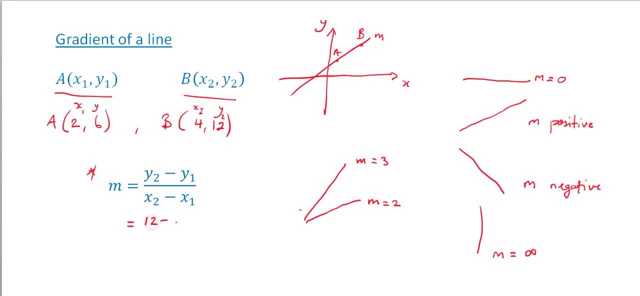 So it's y2 minus y1, so it'll be 12 minus 6 divided by 4 minus 2, and that gives me 6 over 2, which is equal to 3.. So the gradient of the line a b will be equal to 3, right. 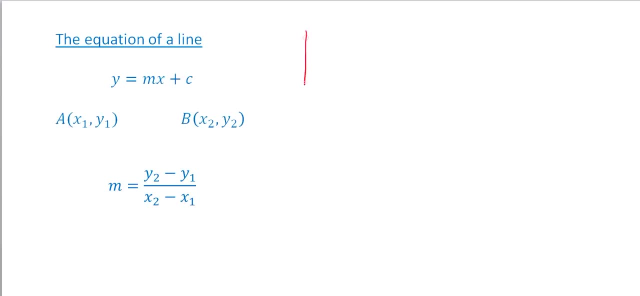 Now, whenever you have a straight line, the equation of any straight line is of the general form: y is equal to 3.. equal to mx plus c, where m is a gradient and c is a coordinate, and it's the y-intercept right. 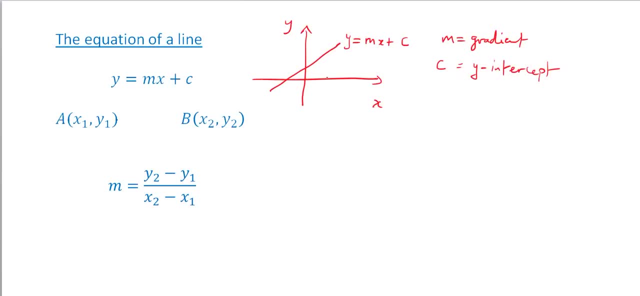 Now, when we say y-intercept, what is the y-intercept? The y-intercept is a point at which a straight line crosses the y-axis. So this point here is the y-intercept, and the coordinate of that y-intercept will be. 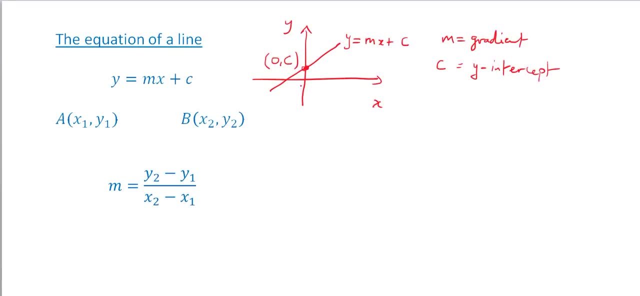 zero c. okay, This is your origin here. So the coordinates of the y-intercept is always zero c, alright. So the general form of the equation of a straight line is: y is equal to mx plus c. So if you see an equation looking like, let's say, y is equal to 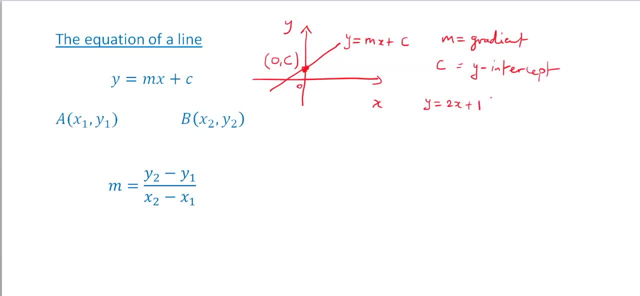 two mx plus c. So if you see an equation looking like, let's say, y is equal to mx plus 1, the gradient of this line is equal to 2, because the coefficient of x is 2 and the y-intercept is zero, 1, right. 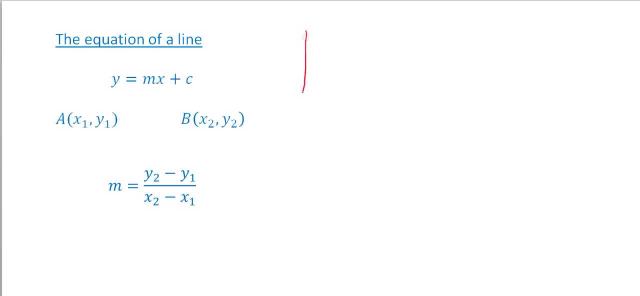 Now, whenever you have a straight line, the equation of any straight line is of the general form: y is equal to 3.. So y is equal to mx plus c, where m is a gradient and c is a coordinate and it's the y-intercept. 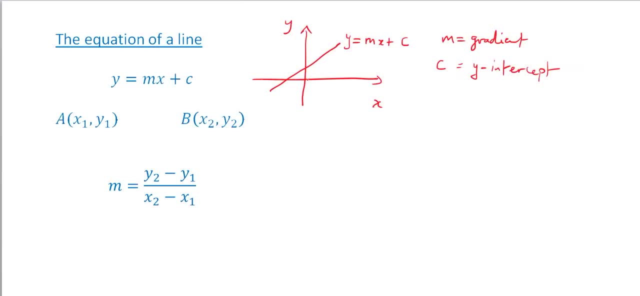 Right Now, when we say y-intercept, what is the y-intercept? The y-intercept is the point at which a straight line crosses the y-axis. So this point here is the y-intercept, and the coordinate of that y-intercept will be 0, c. 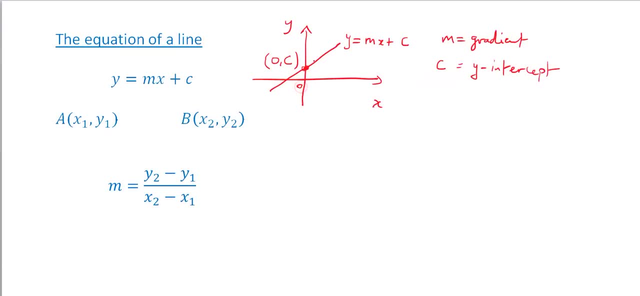 Okay, This is your origin here. So the coordinates of the y-intercept is always 0, c. Alright, So the general form of the equation of a straight line is: y is equal to mx plus c. So if you see an equation looking like, let's say, y is equal to 2x, 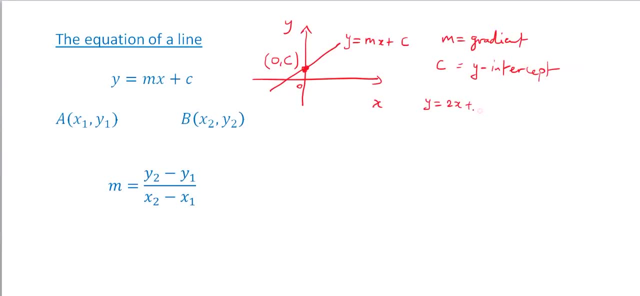 right, So y is equal to 2x plus 1.. The gradient of this line is equal to 2,, because the coefficient of x is 2. And the y-intercept is 0, 1.. Right, So the y-intercept is a point. 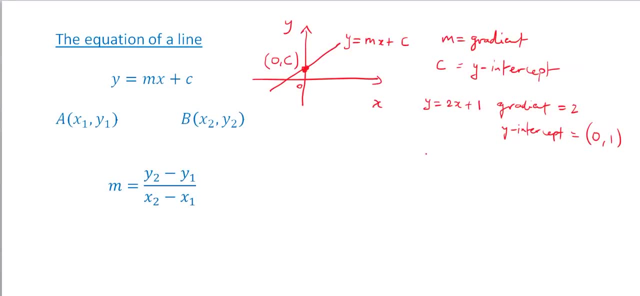 because it has a coordinate, So it's 0, 1.. If we have y is equal to minus 4x plus 2, then the gradient of this line is equal to minus 4, and the y-intercept is equal to. 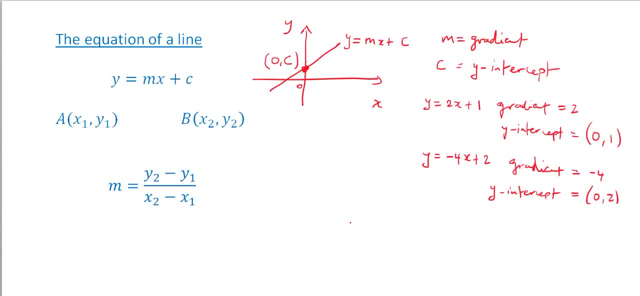 0, 2.. Okay, So, given any two coordinates of points on a straight line, we can find the equation of that straight line by first finding the gradient, which we already know how to find, which is y2 minus y1 over x2 minus x1.. 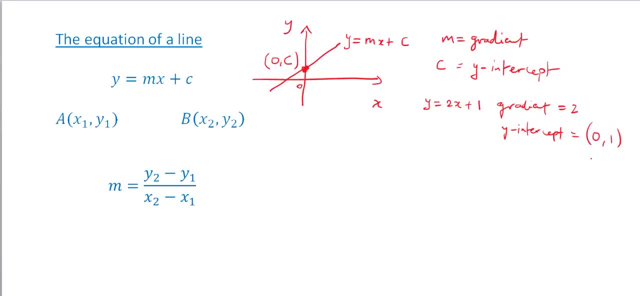 So the y-intercept is a point. therefore it has a coordinate, So it's zero 1.. If we have y is equal to minus 4x plus 2, then the gradient of this line is equal to minus 4 and the y-intercept is equal to zero 2.. 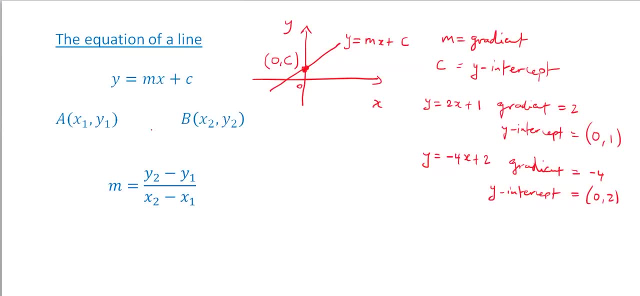 Okay. So given any two coordinates of points on a straight line, we can find the equation of that straight line by first finding the gradient, which we already know how to find, which is y2 minus y1 over x2 minus x1.. 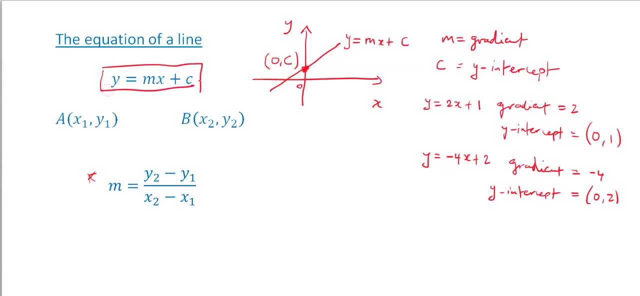 And then we have to get the equation in this form. So let's say we have. let's say a is 2.. Okay, Okay, So we have b, 7, and b is 4,, 13,, and we want to find the equation of the line a- b. 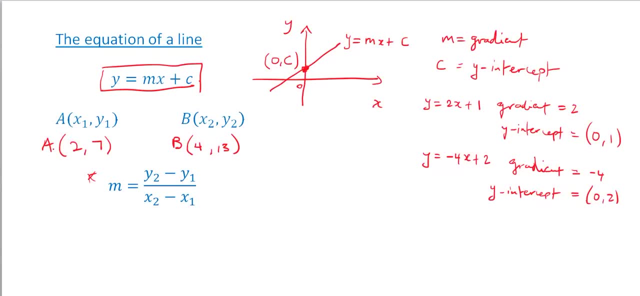 So the first thing we do, we find the gradient. So let's for the coordinates of a, let's call this x1, y1, and let's call this x2, y2.. Okay, Therefore, the gradient will be equal to 13 minus 7,, all over, 4 minus 2,, 13 minus 7 will. 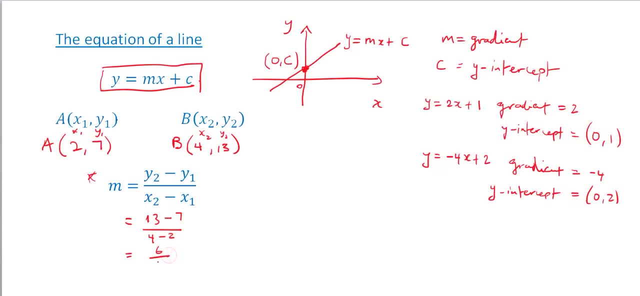 give me 6, and 4 minus 2 is 2,, so the gradient is 3.. Now we have moved out the equation of the line a, b and b. We haven't worked out the equation of the line as yet. we just worked out the gradient. 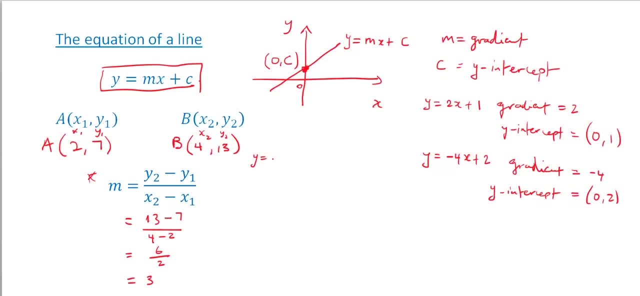 So we know the general form of the equation of a line is equal to mx plus c. So we know what m is. we just worked out m as 3.. So it's y equals 3x plus c. So we haven't worked out the equation completely. we still need to find what c is. 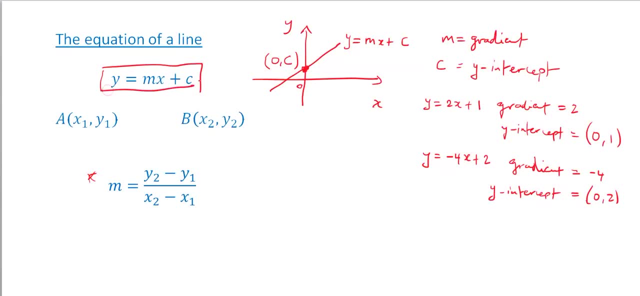 And then we have to get the equation in this form. So let's say we have. let's say a is 2, 7, and b is 4, 13. And we want to find the equation of the line ab. 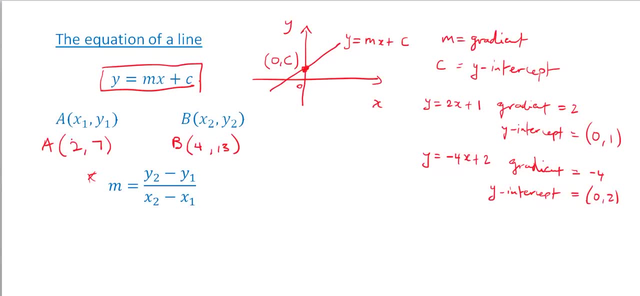 So the first thing we do, we find the gradient. So let's for the coordinates of a, let's call this x1, y1, and let's call this x2, y2.. And therefore the gradient will be equal to. 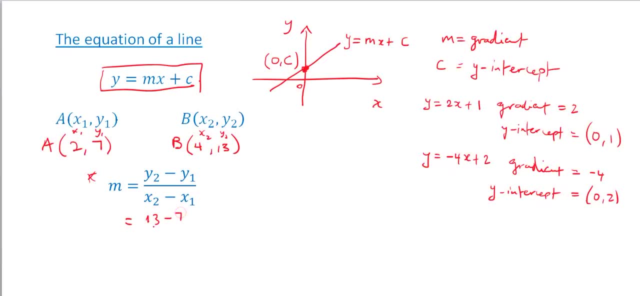 13 minus 7, all over 4 minus 2.. Um, 13 minus 7 will give me 6,, and 4 minus 2 is 2.. So the gradient is 3.. Now we haven't worked out the equation of the line as yet. 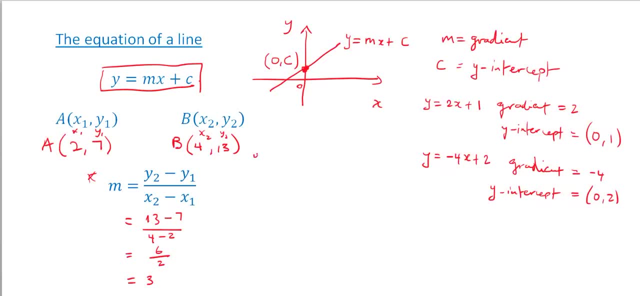 we just worked out the gradient. So we know the general form of the equation of a line is equal to mx plus c. So we know what m is. we just worked out m as 3.. So it's y equals 3x plus c. 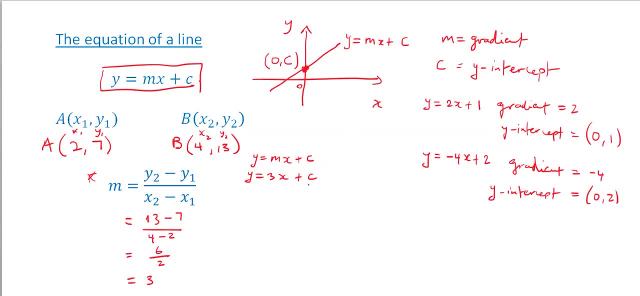 So we haven't worked out the equation completely. we still need to find what c is. So what you do? you choose any one of the two points, a or b. So let's say we choose a, We so using a. 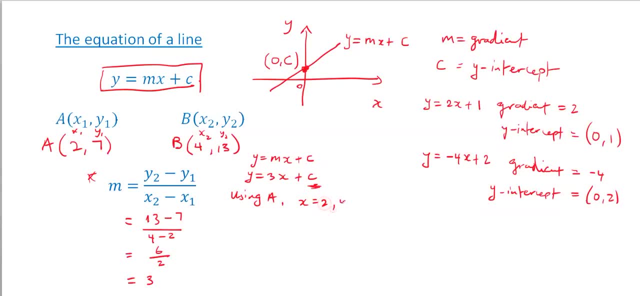 we know that x is equal to 2, and y is equal to 7.. Right, I'm just using the coordinates of a. So therefore, y, which is 7, is equal to 3 multiplied by x, which is 2,. 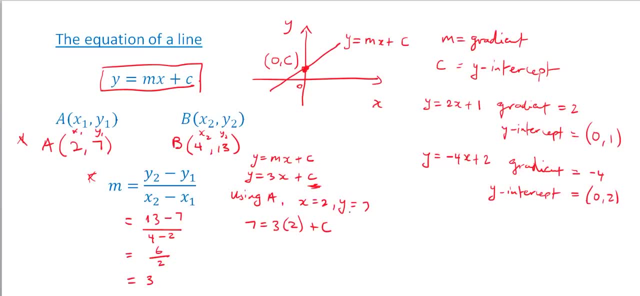 plus c. So what the coordinates of a is allowing me to do is to solve for c. So we have: 7 is equal to 6, plus c, Right? So 7 minus 6 is equal to c. So therefore 1 is equal to c. 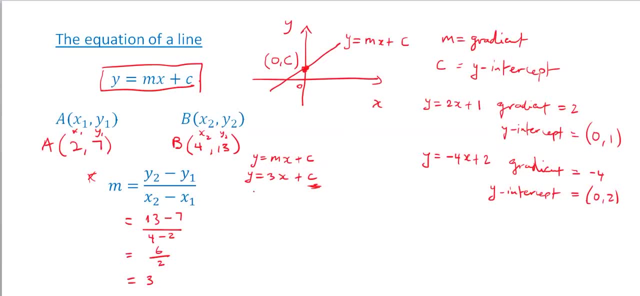 So what you do? you choose any one of the two points, a or b. So let's say we choose a. So, using a, we know that x is equal to 2, and y is equal to 7,. right, I'm just using the coordinates of a. 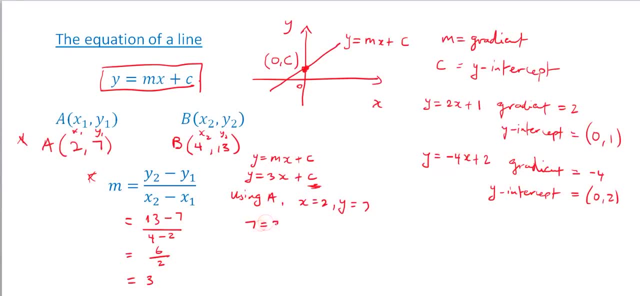 So therefore, y, which is 7, is equal to 3, multiplied by x, which is 2, plus c. So what the coordinates of a is allowing me to do is to solve for c, So we have um, Okay. 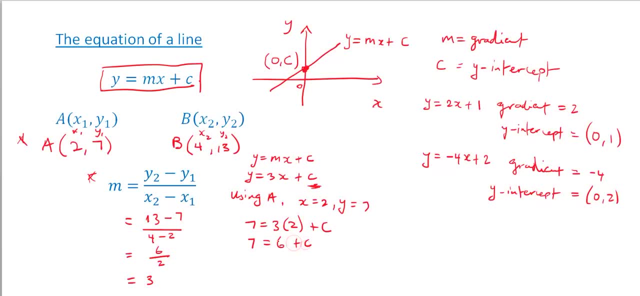 7 is equal to 6, plus c, right? So 7 minus 6 is equal to c. so therefore, 1 is equal to c or c is equal to 1.. So therefore, the final answer, which is the equation of the straight line, will be y is. 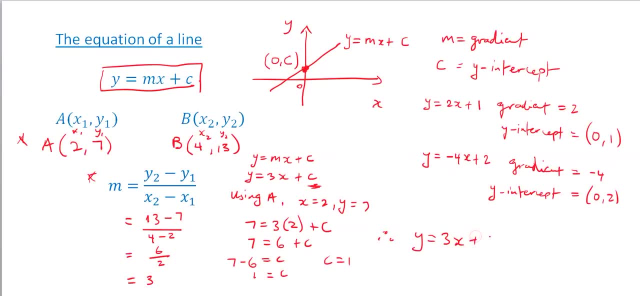 equal to 3x plus 1,. okay, So we worked out the gradient using our formula for gradient, And then we worked out c by using any one of the points a or b into the general form of the equation right. 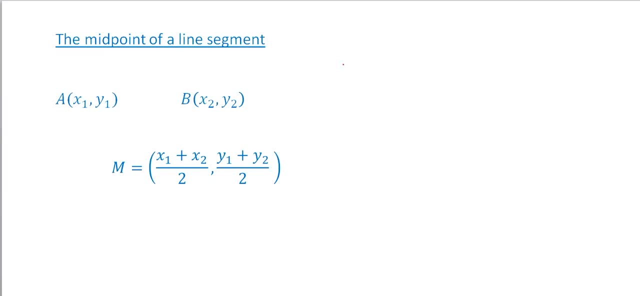 Now we can also find the midpoint of a line segment, which is also pretty straightforward. So if we have two points, a and b, and we wanted to find the midpoint, which is at the middle of the line segment ab, So we have m here, which is the midpoint, and this length is the same as this length. 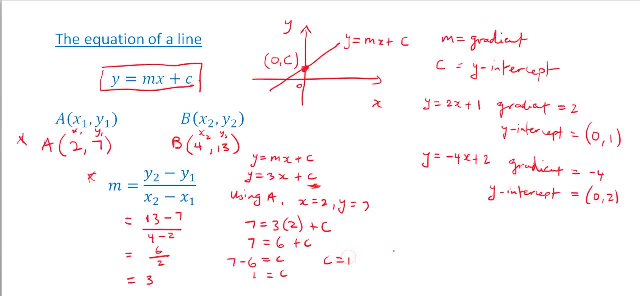 or c is equal to 1.. So therefore, the final answer, which is the equation of the straight line, will be: y is equal to 3x plus c, 1.. Okay, So we worked out the gradient using our formula for gradient. 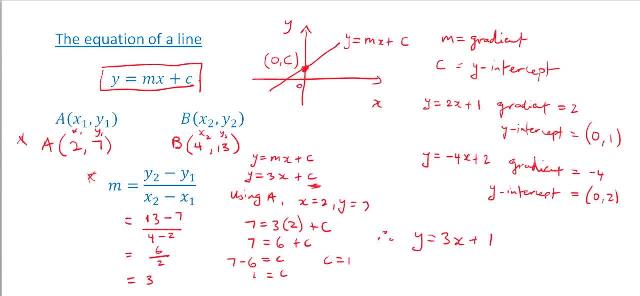 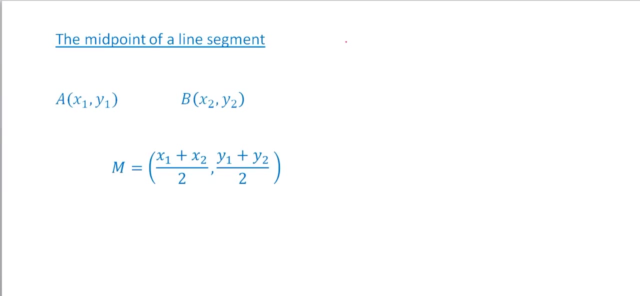 and then we worked out c by using any one of the points a or b into the general form of the equation. Right Now we can also find the midpoint of a line segment, which is also pretty straightforward. So if we have 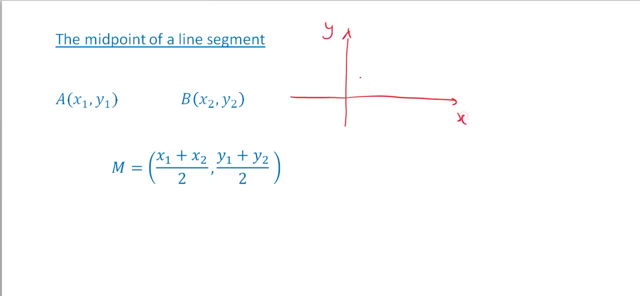 two points, a and b, And we wanted to find the midpoint, which is at the middle of the line segment a- b. So we have m here, which is the midpoint, and this length is the same as this length. 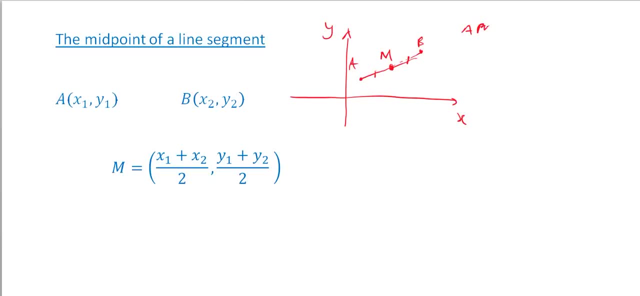 So what we're saying is that a- m is equal to m- b in terms of length, Right, So m is directly in the middle of a and b. How do you get those coordinates? Well, it makes sense. 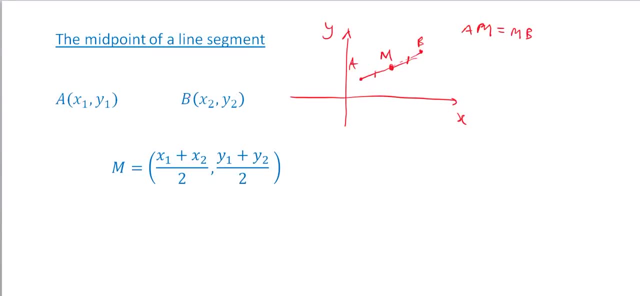 that the midpoint. to find the midpoint, we just add the two x coordinates and divide by two. And we add the two y coordinates and divide by two. But keep in mind that m is a coordinate. So look at how the equation is written. 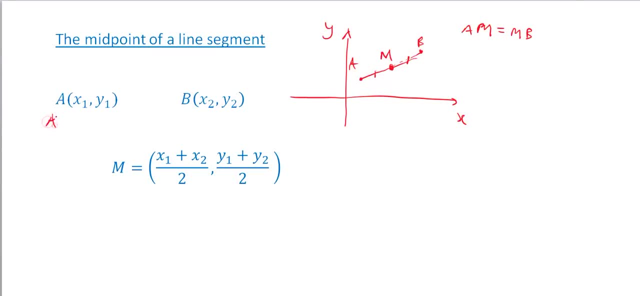 So let's say a is, let's say, three, seven, and b is, let's say, five, nine, And we want to find the midpoint of a- b, Right, If we use the formula just as it is. 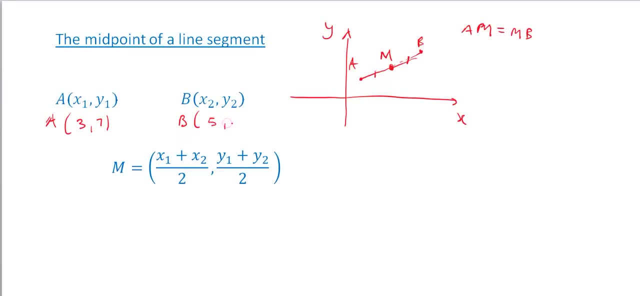 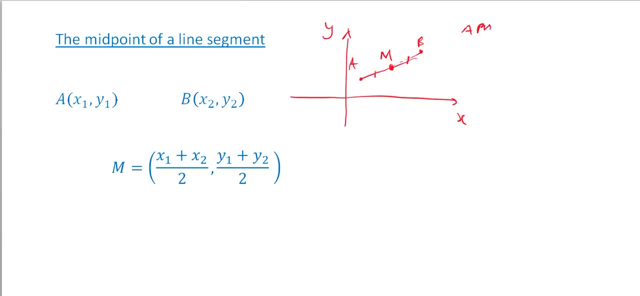 So what we're saying is that am is equal to mb. Okay, In terms of length, right? So m is directly in the middle of a and b. How do you get those coordinates? Well, it makes sense that the midpoint, to find the midpoint, we just add the two x coordinates. 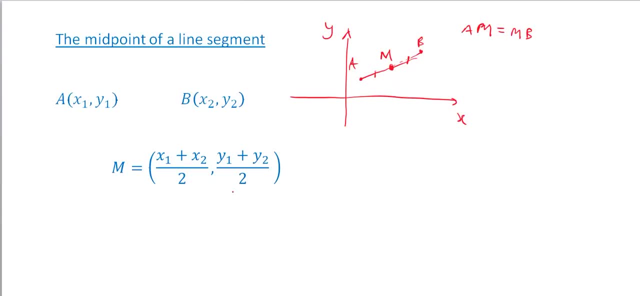 and divide by 2, and we add the two y coordinates and divide by 2.. But keep in mind that m is a coordinate, So look at how the equation is written. So let's say a is, Let's say, Let's say: 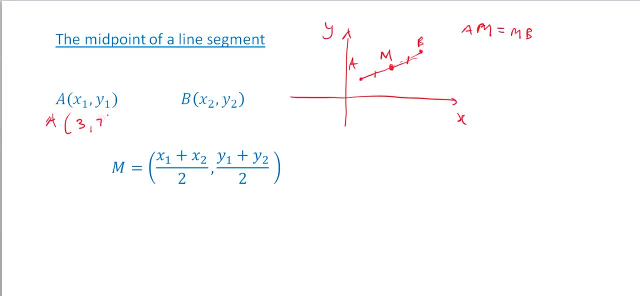 Let's say 3, 7, and b is, let's say, 5,, 9, and we want to find the midpoint of ab right, If we use the formula just as it is, just If you don't want to remember: x1 plus x2 over 2 comma, y1 plus y2 over 2, let's remember. 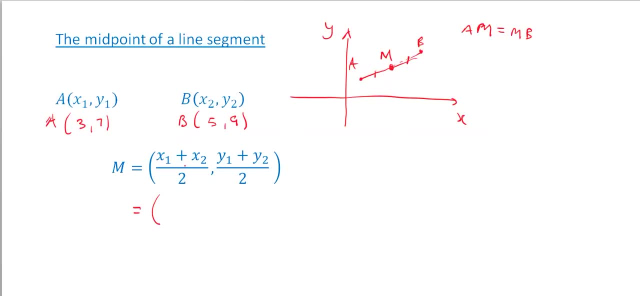 we are adding the two x coordinates and divide by 2.. And we're adding the two y coordinates and divide by 2.. And we're adding the two y coordinates and divide by 2.. Okay, So it will be 3 plus 5, I'm just adding the x coordinates and divide it by 2.. 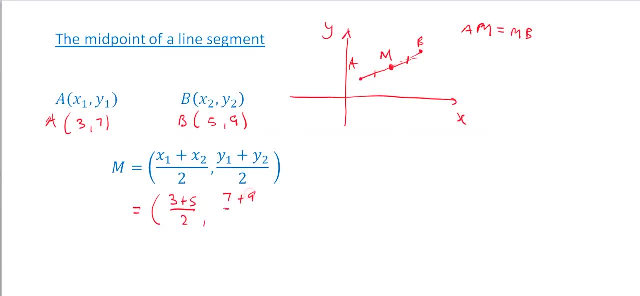 I'm going to add the y coordinates, 7 plus 9, and divide by 2.. So this will be 5, and 3 is 8 over 2,, 9 and 7 is 16 over 2,. therefore the coordinates. 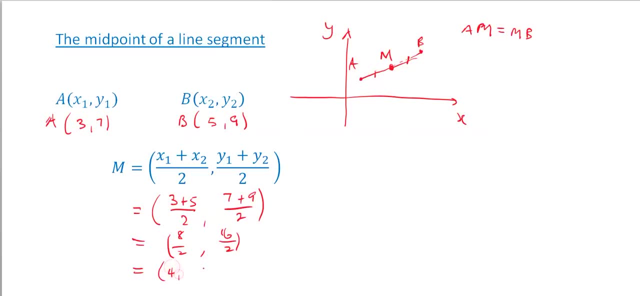 of the midpoint will be: 8 divided by 2 is 4, and 16 divided by 2 is 8.. Right, So this is how you find the midpoint of a line segment. Now, if we have a line segment again and we have a and we have b, we can also be asked: 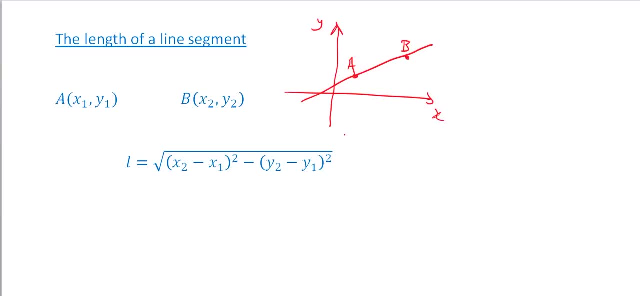 to find the length of the line segment A B. Now, this is just an application of Pythagoras' Theorem, and what we are essentially doing is finding the lengths of this right angle triangle here. So if we are given the coordinates, we can find this length, and we can also find this. 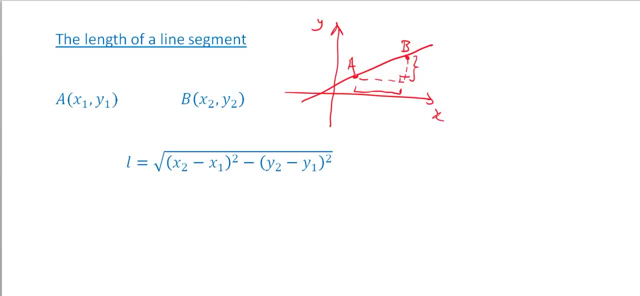 length and we just use Pythagoras' Theorem to find the length A- B. So if you look at this line segment, you can see that this is the length of the line segment. Okay, So if we look at the equation which is here- you need to remember this- it looks very similar. 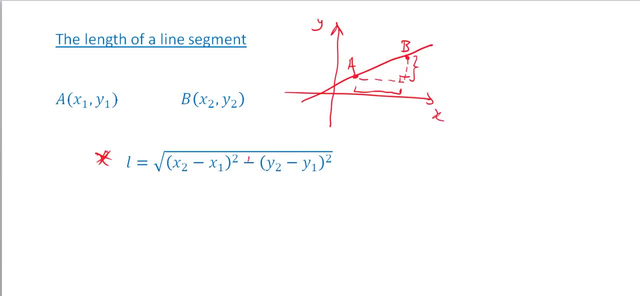 to Pythagoras' Theorem, And this is a mistake. this is supposed to be plus right. So let me give you an example. So let's say E is 2, 4, and B is 3, 6.. 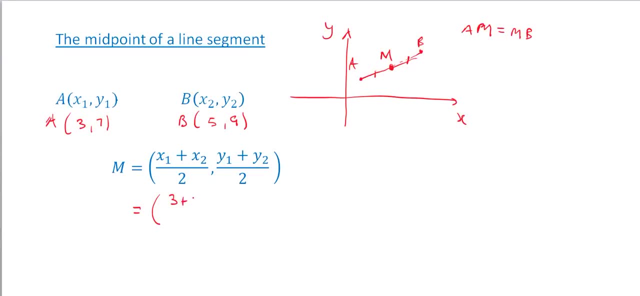 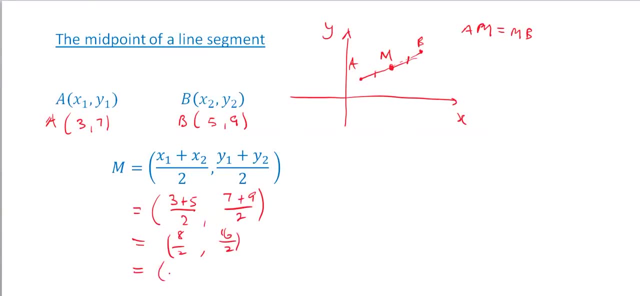 Therefore, the coordinates of the midpoint will be: 8 divided by 2 is 4, and 16 divided by 2 is 8.. So this is how you find the midpoint of a line segment. Now, if we have a line segment again and we have A and we have B, we can also be asked: 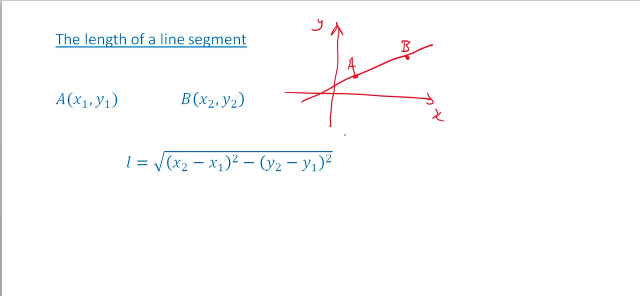 to find the length of the line segment AB. Now, this is just an application of Pythagoras' Theorem, and what we are essentially doing is finding the lengths of this right angle triangle here. So if we are given the coordinates, we can find this length, and we can also find this. 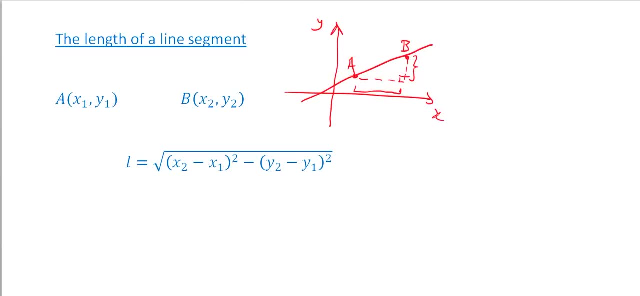 length and we just use Pythagoras' Theorem to find the length AB. So if you look at the equation which is here- you need to remember this- it looks very similar to Pythagoras' Theorem And this is a mistake. this is supposed to be plus right. 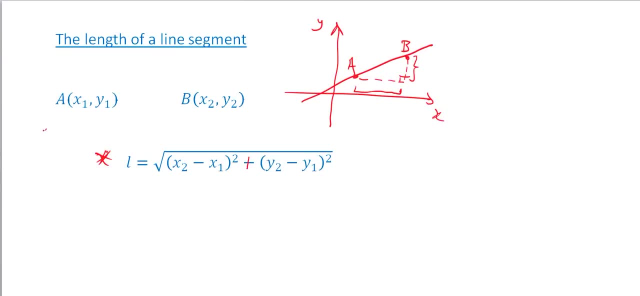 So let me give you an example. So let's say A is 2, 4 and B is 3, 6, right? So the length of the line segment AB will be the difference of the two X values. So, like I said, you need to label. 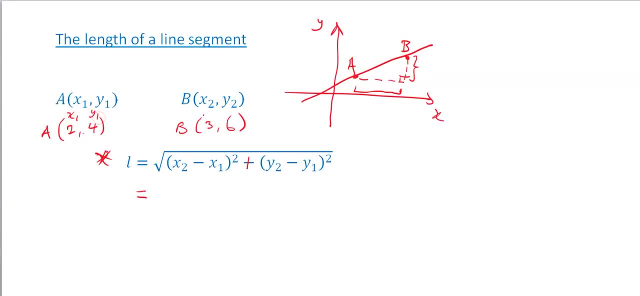 Which one? Which one is X1?? So X1, Y1,, X2, Y2.. Now, I can tell you that this is very important. When I started maths a long time ago, this is what I used to do, right. 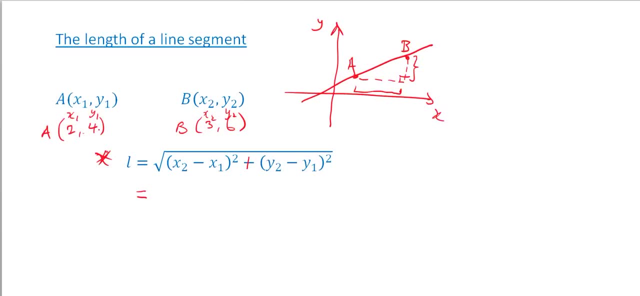 So that I do not get confused. So you need to label X1, Y1 and X2, Y2 and you need to be consistent. So you kind of put X1, Y2 here and then you reverse on the other side. 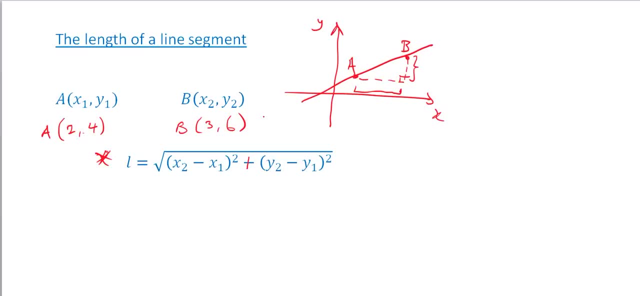 Okay, So the length of the line segment A, B will be the difference of the two x values. So, like I said, you need to label which one is x1,. so x1, y1, x2, y2.. Now I can tell you that this is very important. 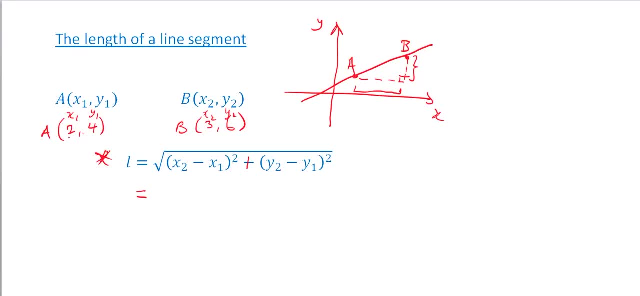 When I started maths a long time ago. this is what I used to do, right, So that I do not get confused. So you need to label x1, y1, and x2, y2.. Okay, And you need to be consistent. 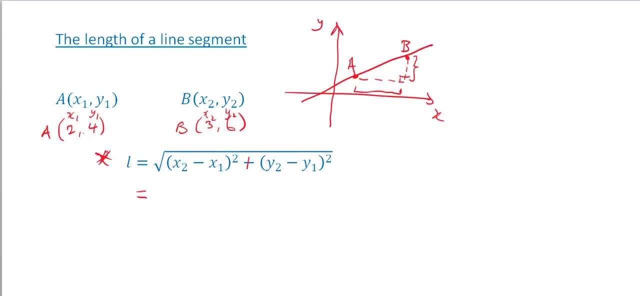 So you kind of put x1, y2 here and then you reverse on the other side. Be very careful with that, because you can make a mistake very easily. Okay, So x2 minus x1, so this will be 3 minus 2 squared plus the difference in y, which is: 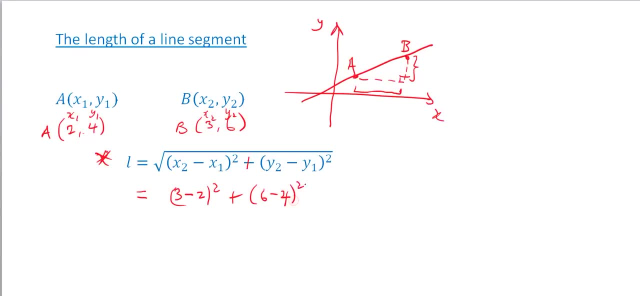 6 minus 4 squared, and we're going to find the square root of all of this. So 3 minus 2.. 2 is 1, so this is 1 squared. plus 6 minus 4 is 2, so this is 2 squared. again, we find: 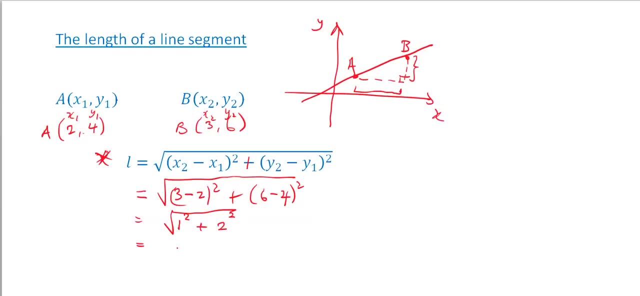 the square root, And this will be 1 plus 2, 2 is 4, so this will be the square root of 5 units, And the reason why we put in units is because we're finding the length of a line segment. 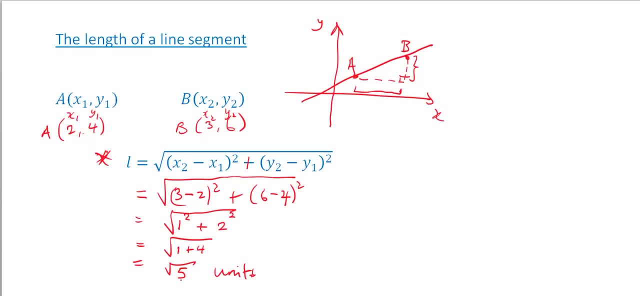 Okay, So you can use a calculator and find the square root of 5, all right, which would be 2 point something, or you can leave the answer as the square root of 5.. Okay, Now let's talk a little bit about parallel and perpendicular lines. 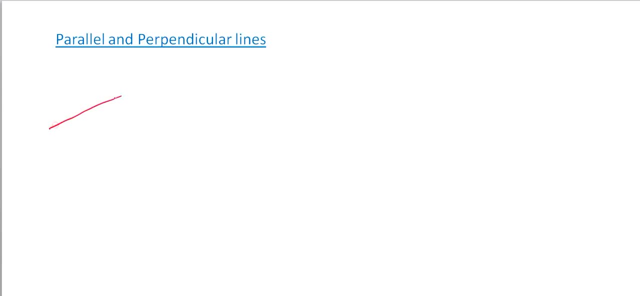 So what are parallel lines? Suppose we have two lines, This is A, B, Okay, And we have another line, which is C, D. Now, these two lines, A, B and C, they are parallel, meaning that if we extend them to infinity, as in, we keep drawing in this direction here. 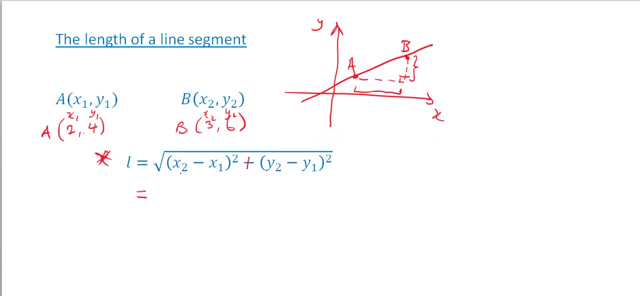 Be very careful with that, because you can make a mistake very easily. Okay, So X2 minus X1, so this will be 3 minus 2 squared, plus the difference in Y, which is 6 minus 4 squared, and we're going to find the square root of all of this. 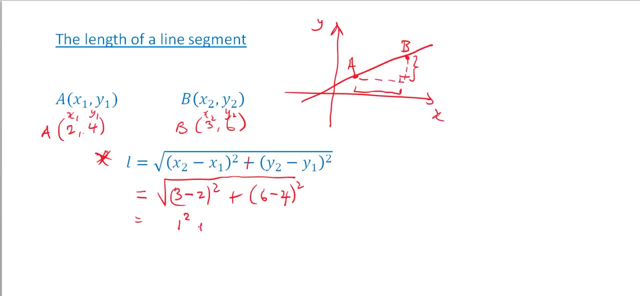 So 3 minus 2 is 1, so this is 1 squared. plus 6 minus 4 is 2,, so this is 2 squared. Again, we find the square roots Okay And this will be 1 plus 2, 2 is 4.. 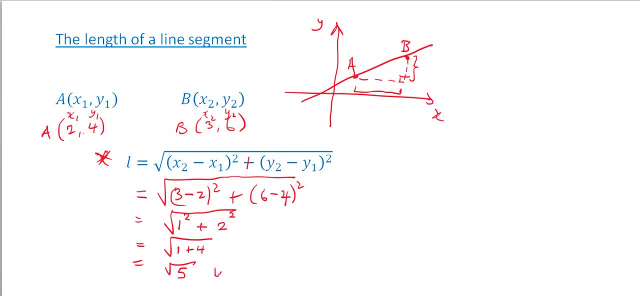 So this will be the square root of 5 units, and the reason why we are putting units is because we're finding the length of a line segment. Okay, So you can use a calculator and find the square root of 5, right, which would be 2, point something. 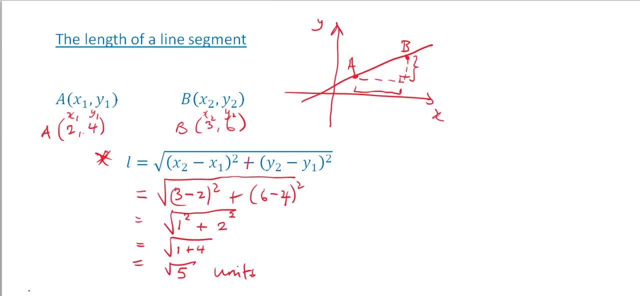 or you can leave the answer as the square root of 5.. Okay, Now let's talk a little bit about parallel and perpendicular lines. So what are parallel lines? Suppose we have two lines: this is AB and we have another line which is CD. 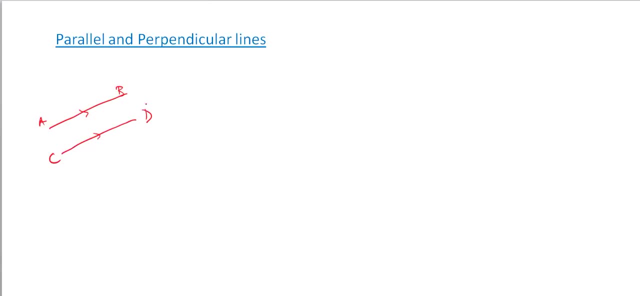 Now these two lines, AB and CD, are parallel, Okay, But if we extend them to infinity, as in we keep drawing in this direction here, they will never meet. So parallel lines never meet right on a plane surface. So what do we need to know about parallel lines? 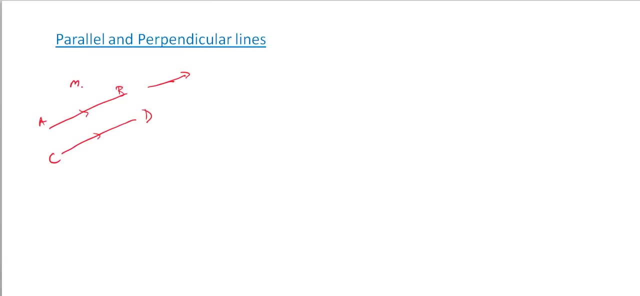 If the gradient of one of them is M, let's say one of them is the gradient is 2, then the gradient of the other one must also be 2.. So for parallel lines, they have the same length, They have the same gradient. 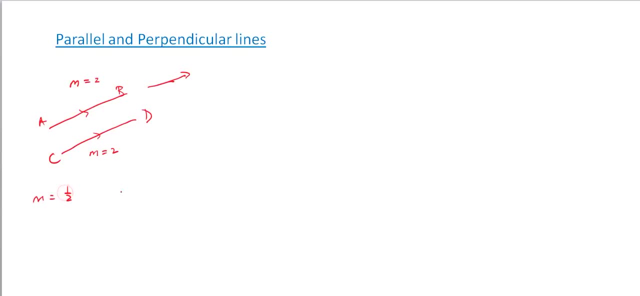 So if one of them was half, then the second one will also be a half, right Now in the case of perpendicular lines, though. so let's say we have a line AB and we draw another line. Okay, So let's say we have a line AB. 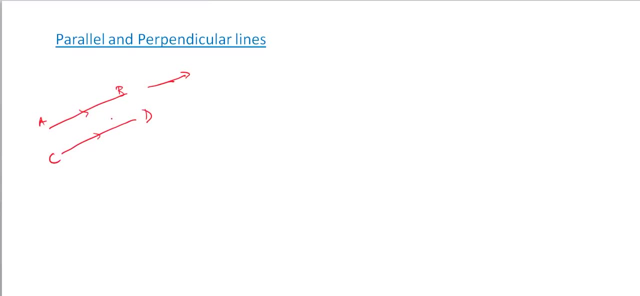 they will never meet. So parallel lines never meet right on a plane surface. So what do we need to know about parallel lines If the gradient of one of them is m squared? Okay, Let's say one of them is the gradient is 2, then the gradient of the other one must. 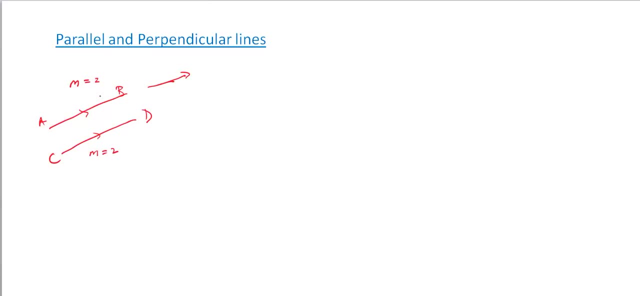 also be 2.. So for parallel lines they have the same gradient, So if one of them was half, then the second one will also be a half, right Now in the case of perpendicular lines though. So let's say we have. 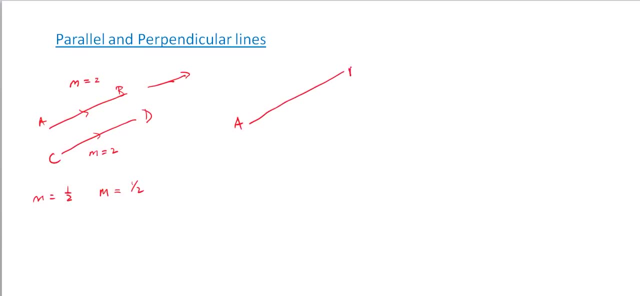 Okay, Let's say we have a line A- B and we draw another line, C- D, and they are 90 degrees to each other, right? So they are at right angles. So A- B is perpendicular to C- D, right? 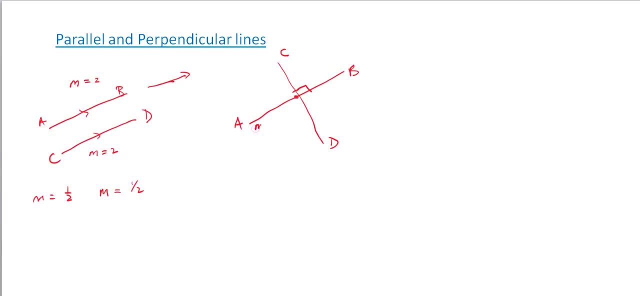 What can we say about the gradients? So if the gradient of A- B is m1, and the gradient of C- D is m2,, the relationship between the two of them are as follows: the gradient of 1 multiplied by the gradient of the second. 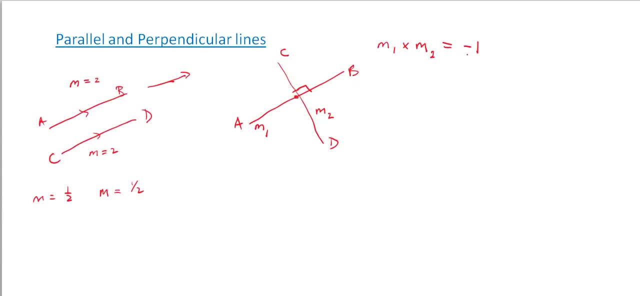 one is equal to minus 1.. So therefore, if one line, so let's say A, B, the gradient was 2, and therefore the gradient of m2 has to be minus 1.. Okay, Then the gradient of A- B is a half, in order for us to get minus 1.. 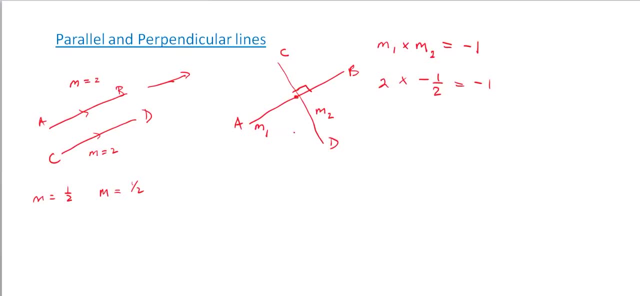 So you can be given the gradient of one line and you will be asked to find the gradient of a line that is perpendicular to it, right? So let's say we have a line and they tell you that the gradient of one line is: let's. 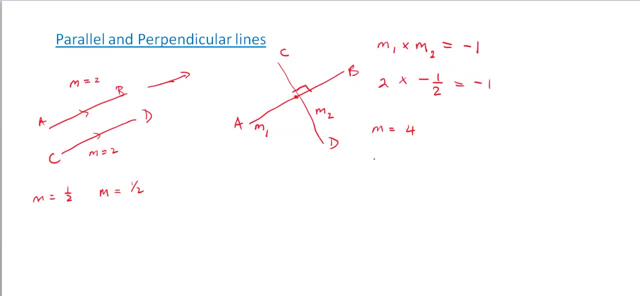 say 4. Then the gradient of the line that is perpendicular to that line will be. All you have to do is put a minus sign in front and invert the gradient right. So the gradient of the other line will be minus a quarter. okay. 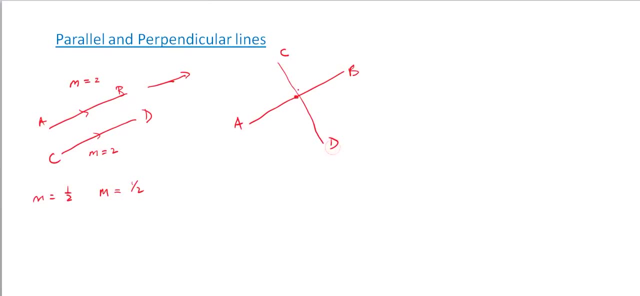 Okay, So let's say we have a line CD and they are 90 degrees to each other, right? So they are at right angles. So AB is perpendicular to CD, right? What can we say about the gradients? So if the gradient of AB is M1 and the gradient of CD is M2, the relationship between the 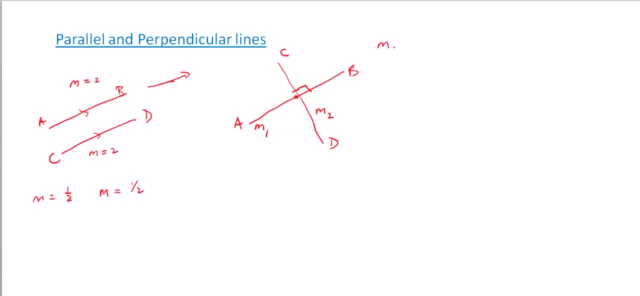 two of them are as follows: The gradient of 1 multiplied by the gradient of CD Of the second one is equal to minus 1.. So therefore, if one line, so let's say AB, the gradient was 2, and therefore the gradient 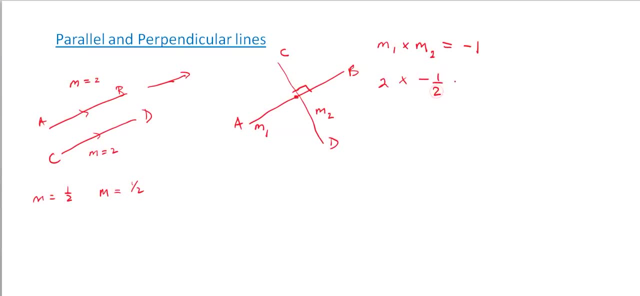 of M2 has to be minus a half in order for us to get minus 1.. So you can be given the gradient of one line and you will be asked to find the gradient of a line that is perpendicular to it, Right? So let's say we have a line and they tell you that the gradient of one line is: let's. 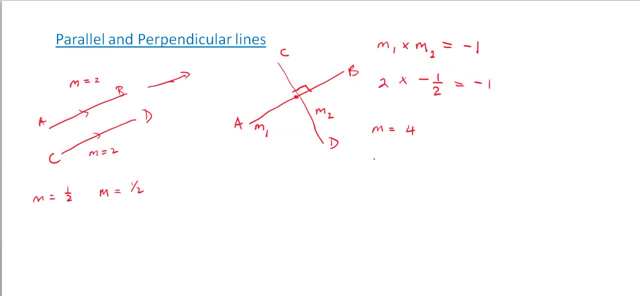 say 4. Then the gradient of the line that is perpendicular to that line will be: you have to. all you have to do is put a minus sign in front and invert the gradient right, So the gradient of the other line will be minus a quarter. 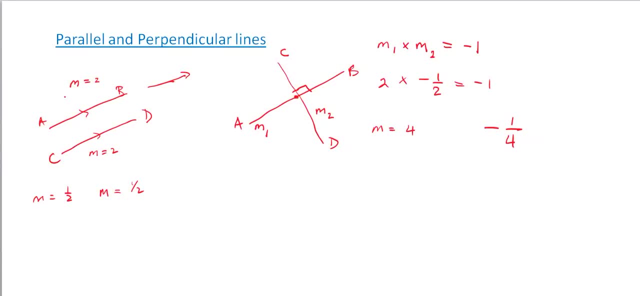 Okay, And if you come to that question, Okay, I'm going to say this now, A little thing you need to know as well. You can be given the equation of a line, let's say Y is equal to 4 minus 2X, and you want 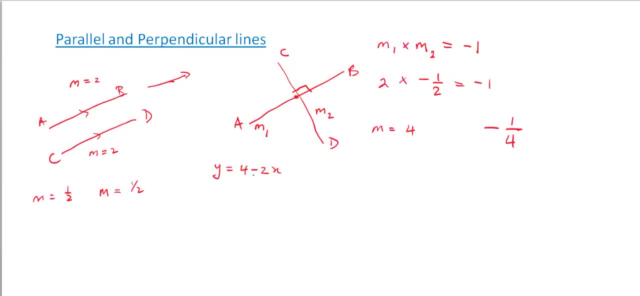 to know what is the gradient of the line. So just by looking at this line, the gradient has to be minus 2, right? Even though the general equation of a straight line is Y equal MX plus CD, You may be given an equation that looks a little strange. 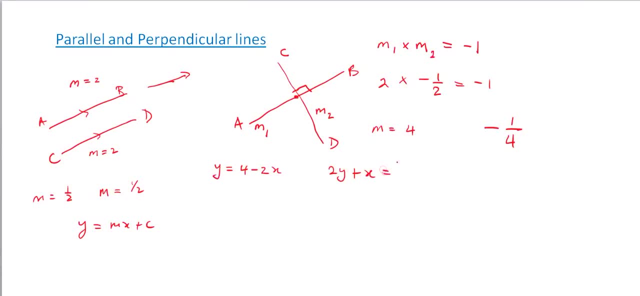 So you might see 2Y plus X is equal to, let's say, 4, and you have to look at this line and figure out what the gradient is. So the first thing you have to do is to write this equation in the form: Y equal MX plus. 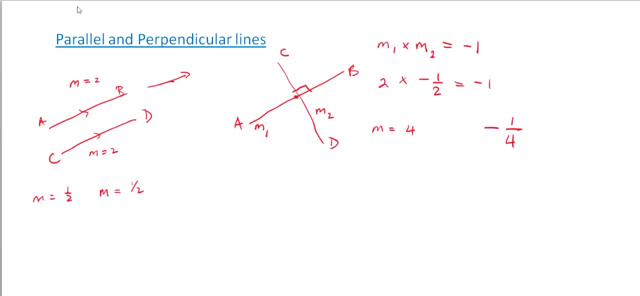 And we'll come to that question just now. A little thing you need to know as well. You can be given the equation of a line. let's say y is equal to 4 minus 2x. Okay, Let's say y is equal to 2x. 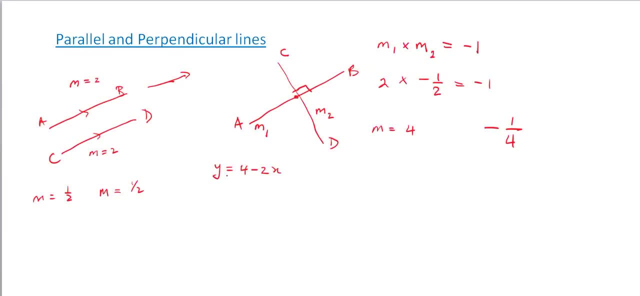 Okay, And you want to know what is the gradient of the line. So just by looking at this line, the gradient has to be minus 2, right? Even though the general equation of a straight line is y equal mx plus c, you may be given. 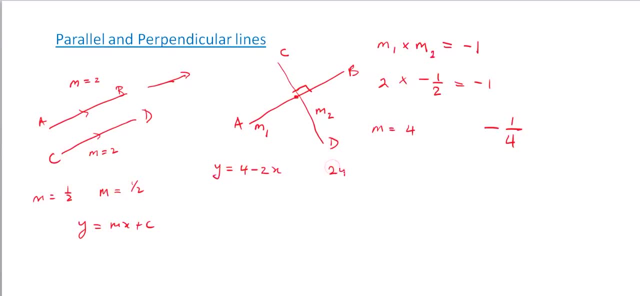 an equation that looks a little strange. So you might see 2y plus x is equal to, let's say, 4, and you have to look at this line and figure out what the gradient is. Okay, So the first thing you have to do is to write this equation in the form: y equal mx plus. 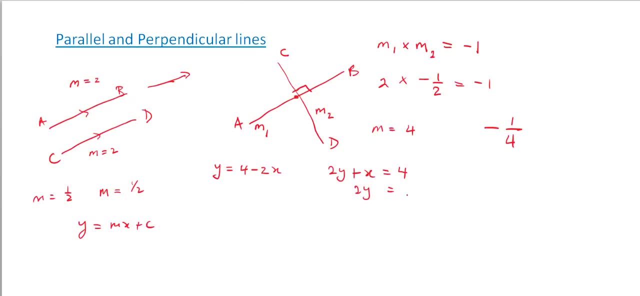 c. So we can write: 2y is equal to minus x plus 4.. All I did was move the x to the right-hand side and therefore y you divide everything by 2, is equal to minus x over 2, plus 4 over 2.. 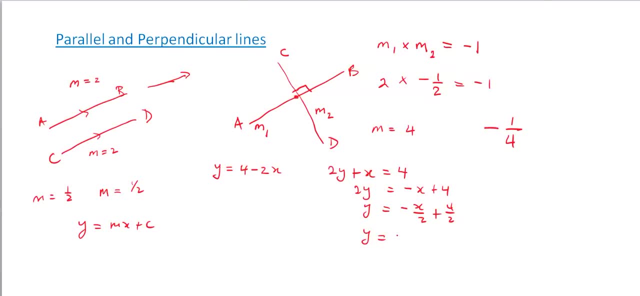 And this can be written as minus 2y. Okay, Okay, So now we have 1.5x plus 2.. So therefore, the gradient of this line is equal to minus 1.5.. All right, So if you just looked at this equation here, you can't just look at it and say, well, oh, 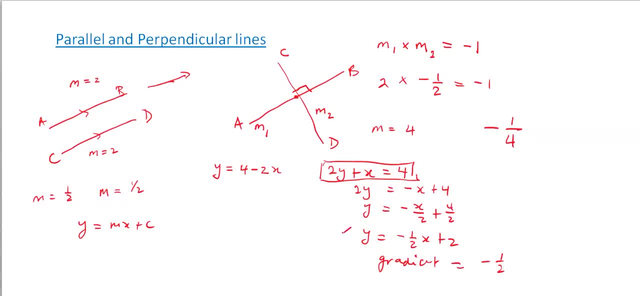 the gradient is 1.. You must write it in the form: y is equal to mx plus c, which is what we did here, and then identify what is the gradient. Okay, So let me do another example. Okay, So if you have, let's say, 2y minus 8x equal 1, and we want to find the gradient of this, 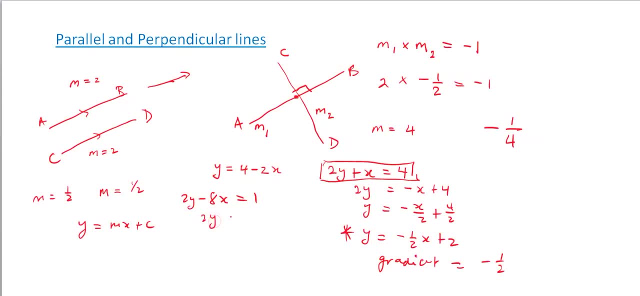 line, so we have to write it in the form y equal mx plus c, So 2y is equal to 8x plus 1.. All I did was move the minus 8x to the right-hand side and I need to divide everything by 2.. 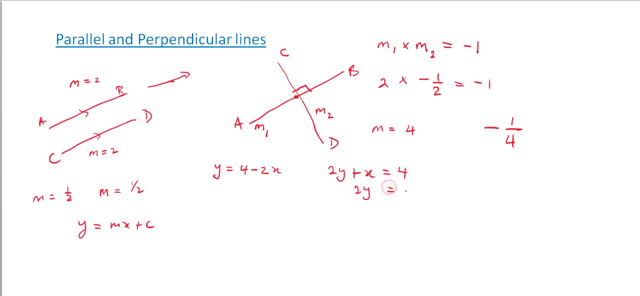 C, So we can write: 2Y is equal to minus X plus 4.. All I did was move the X to the right hand side. Okay, And therefore Y you divide everything by 2, is equal to minus X over 2 plus 4 over. 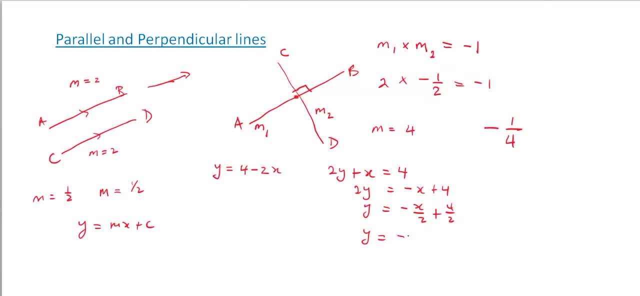 2.. And this can be written as minus half X plus 2.. So therefore, the gradient of this line is equal to minus half, right? So if you just looked at this equation here, You can't just look at it and say, well, oh, the gradient is 1.. 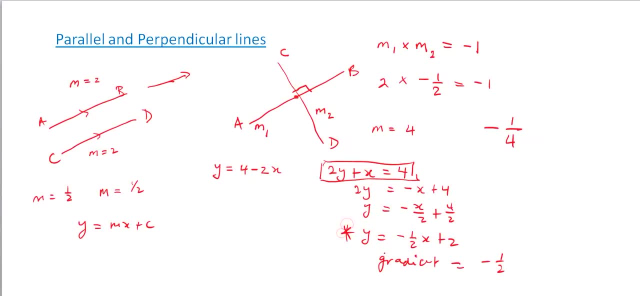 You must write it in the form: Y is equal to MX plus C, which is what we did here, And then identify what is the gradient. Okay, So let me do another example. So if you have, let's say, 2Y minus 8X equal 1.. 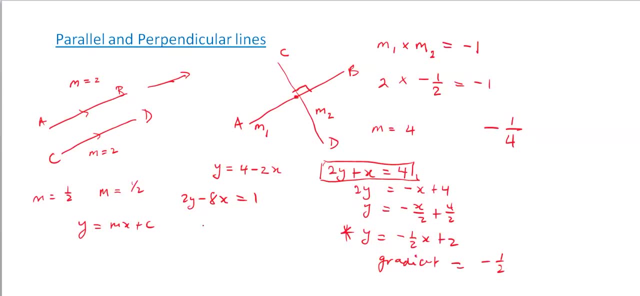 And we want to find the gradient of this line. So we have to write it in the form Y equal MX plus C. So 2Y is equal to 8X plus 1.. All I did was move the minus 8X to the right hand side. 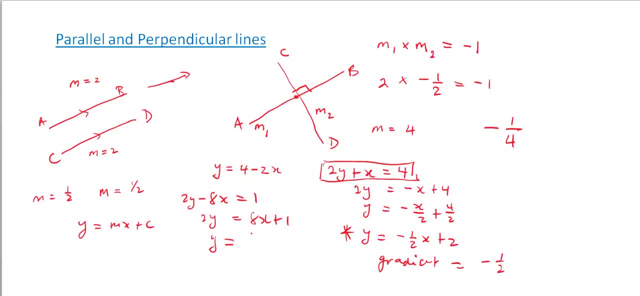 And I need to divide everything by 2.. So this will be 8X over 2 plus 1 over 2.. Therefore, Y is equal to 4X plus a half. Okay, So this will be 8X over 2 plus 1 over 2.. 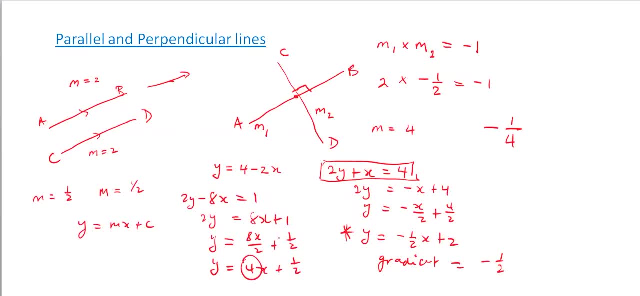 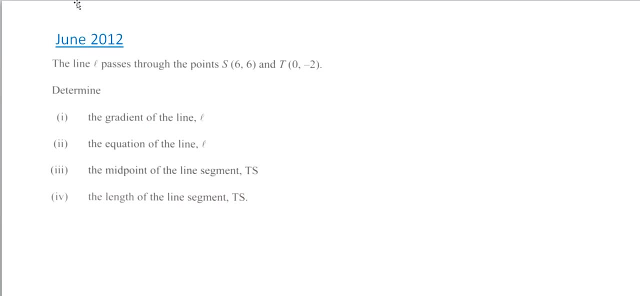 Therefore, Y is equal to 4X plus a half. All right, So the gradient in this case is 4.. All right, So let's look at an example now. This is from the June 2012 paper. They tell you, a line passes through the points S, which is 6,, 6,, and the point T, which 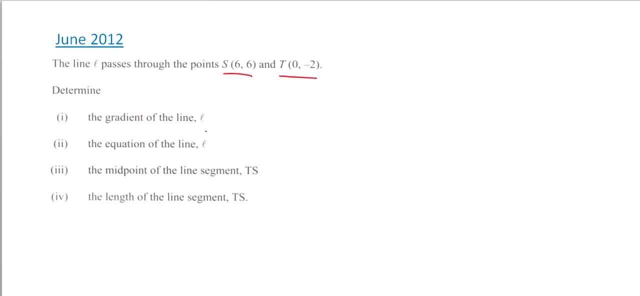 is 0 minus 2.. And the first thing they want to find is the gradient of the line. So the first thing we need to do is to label our X1., Y1, X2, Y2.. Now, I'm very serious about this. 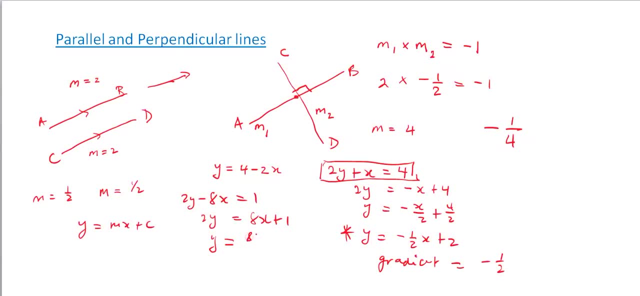 So 2y is equal to 8x plus 1.. So this will be 8x over 2 plus 1 over 2, and for y is equal to 4x plus 1.5,. all right, So the gradient in this case is 4,. all right. 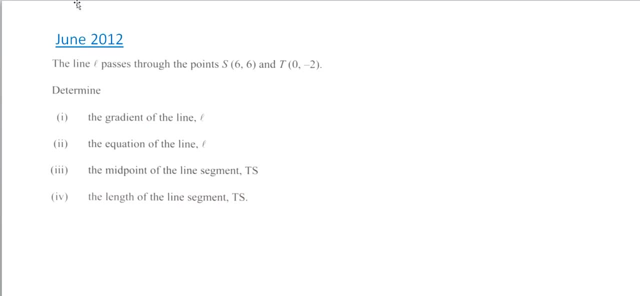 So let's look at an example now. This is from the June 2012. people, and they tell you, a line passes through the points s, which is 6.5.. All right, So this is 6, 6, and the point t, which is 0 minus 2, and the first thing they want to. 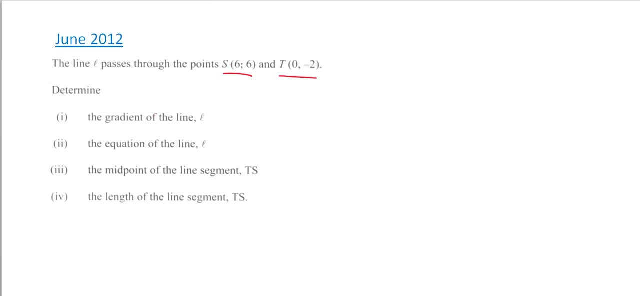 find is the gradient of the line. So the first thing we need to do is to label our x1, y1, x2, y2.. Now, I'm very serious about this. You need to label your points, please. In the exam paper you can write these: write: x1 and y1, x2, y2.. 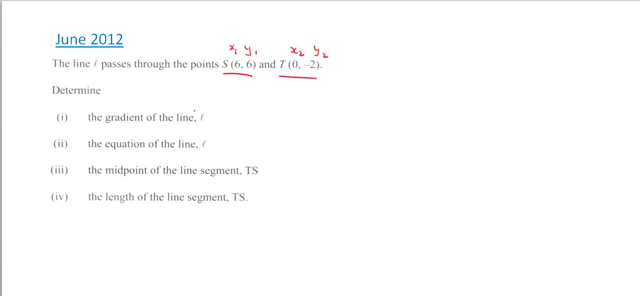 If you do that then you will not make a mistake, All right. So the first part: find the gradient of the line. So if you know gradient m, let me do it on this side here. Gradient m is equal to difference in y, which is y2 minus y1, over x2 minus x1, all right. 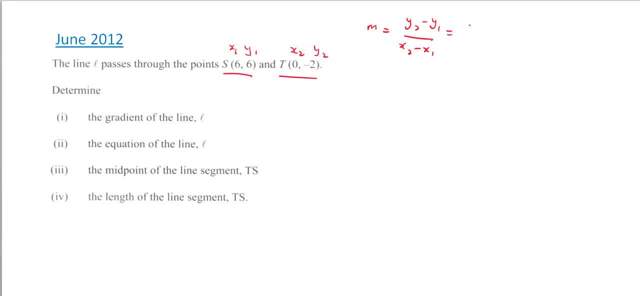 So just by looking at how we label it now, y2, which is minus 2,, minus 6,, all over 0, x1.. You see, if I label my points, there's no way I'll make a mistake when I substitute. 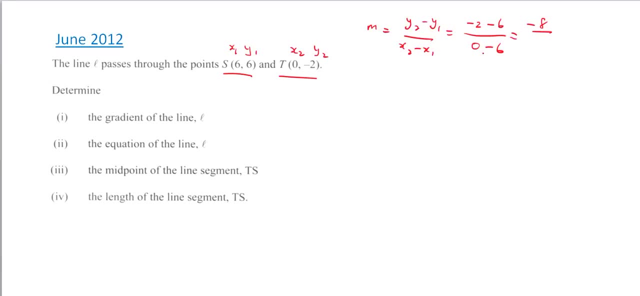 Minus 2 minus 6 is minus 8, and 0 minus 6 is minus 6,, and this will give me 4 over 3.. So the gradient is 4 over 3,. all right, The next thing they want to know: what is the equation of the line? 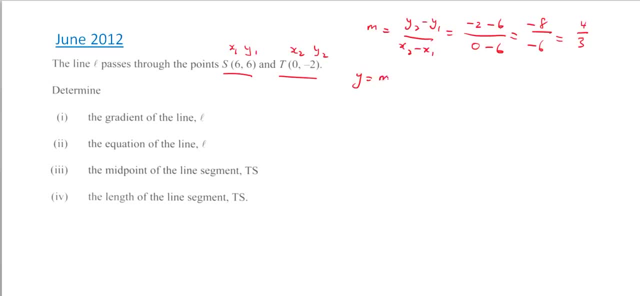 So we know the general equation of a line. The general equation of a line is y equal mx plus c. We already know the gradient. The gradient is 4 over 3.. So therefore y is equal to 4 over 3x plus. sorry, this is c here. 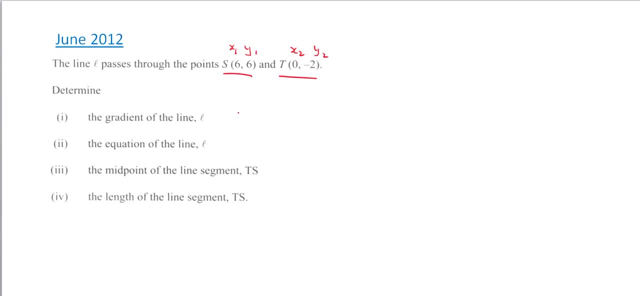 You need to label your points, please. In the exam paper you can write X1 and Y1,, X2, Y2.. If you do that, then you will not make a mistake. All right, So the first part: find the gradient of the line. 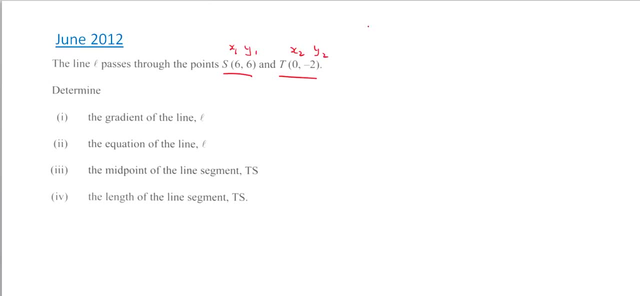 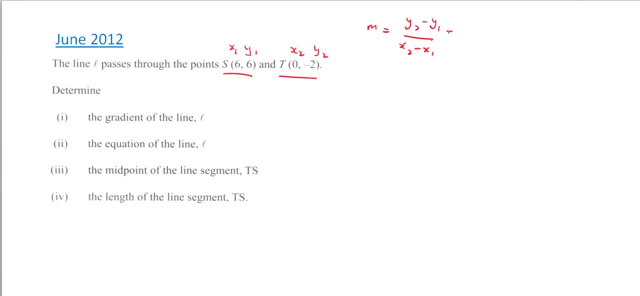 All right, X2 minus X1.. All right, So just by looking at how we label it now, Y2, which is minus 2, minus 6, all over, 0 minus 6.. All right, You see, if I label my points, there's no way I'll make a mistake when I substitute. 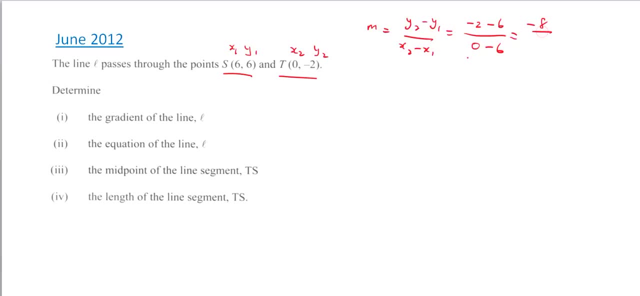 Minus 2 minus 6 is minus 8.. And 0 minus 6 is minus 8.. That's 6.. And this will give me 4 over 3. So the gradient is 4 over 3.. All right. 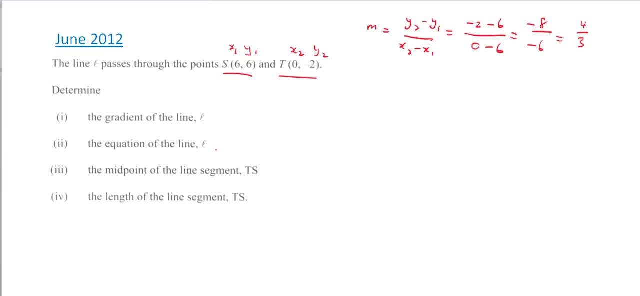 Next thing, they want to know what is the equation of your line. So we know. the general equation of a line is: Y equals MX plus C. We already know the gradient. The gradient is 4 over 3.. So therefore, Y is equal to 4 over 3.. 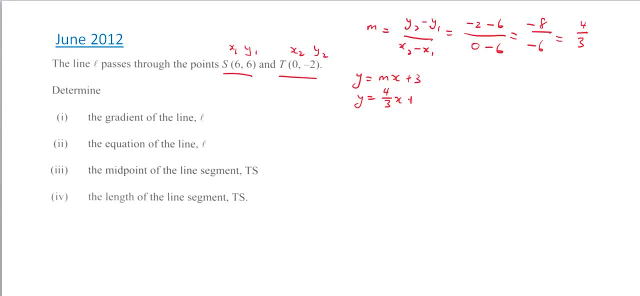 OK, OK, x plus sorry, this is c. here y is equal to 4 over 3x plus c. so what we do? we take any one of the points. so i'm going to use t, right, because the numbers are smaller to work with. all right. so 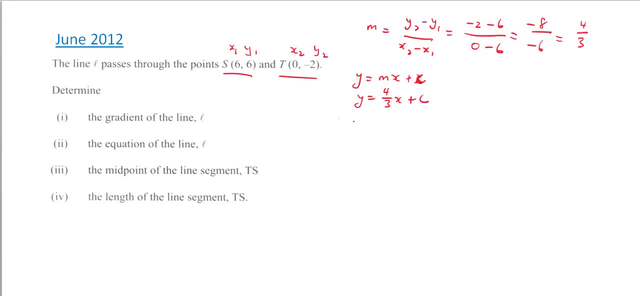 i'm using a point t, we can say that y, so t is really 0 minus 2. what does this tell me? it tells me that when x is equal to 0, y is equal to minus 2, so therefore minus 2 is equal to 4. x over 3. 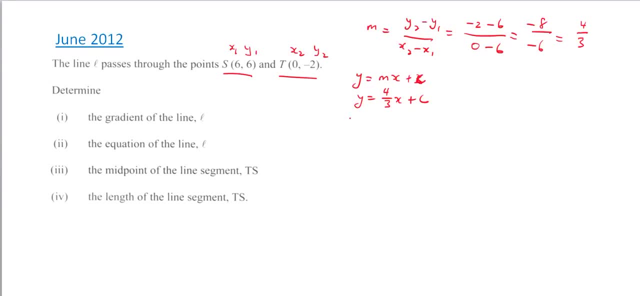 y is equal to 4 over 3x plus c. So what we do? we take any one of the points. So I'm going to use t, all right, because the numbers are smaller to work with, All right. So if I use any point t, we can say that y, so t is really 0 minus 2.. 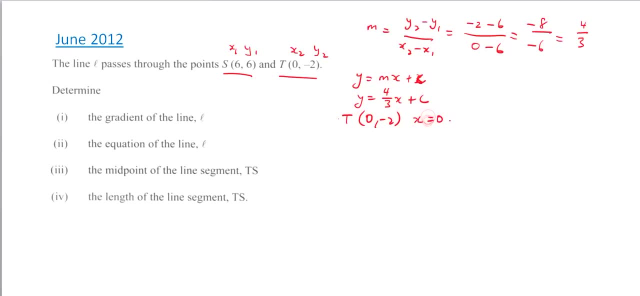 What does this tell me? It tells me that when x is equal to 0, y is equal to minus 2.. So, therefore, minus 2 is equal to 4x over 3 plus c, which is minus 2.. Sorry. 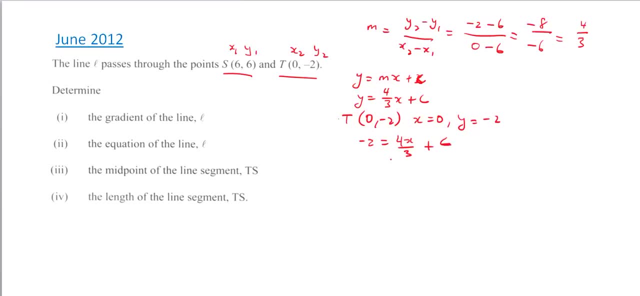 What am I doing? Plus c: All right. So now what we should do is to get rid of this tree at the bottom here. So we multiply everything by 3. And this will give me: minus 6 is equal to 4,. sorry, I made a mistake here. 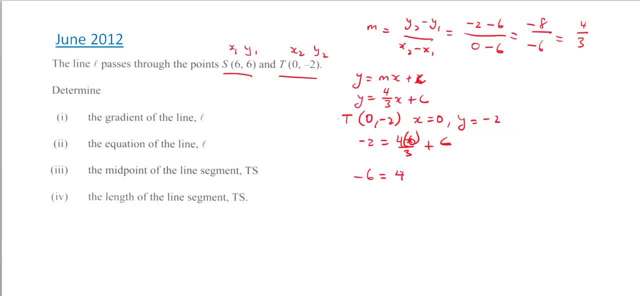 This is 0,. all right, So this will give me sorry. I don't even need to do that. This has minus 2.. And this will be 0 plus c. Sorry about that. So therefore, minus 2 is equal to c, all right. 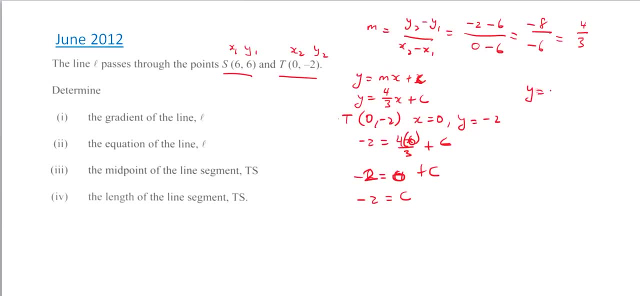 So, therefore, the equation of the line will be: y is equal to 4 over 3x minus 2, all right, So this is the answer for the first part. This is the final answer for the second part, That is, the equation of the line. 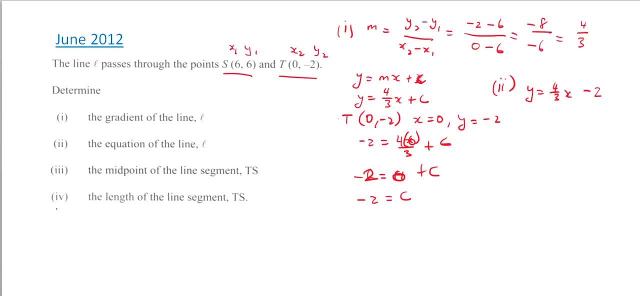 But I want the midpoint of the line, segment ts, So let me work out midpoint. So midpoint m is equal to: I have to add x1 plus x2 over 2, comma y1 plus y2 over 2.. So we're going to add the two x-coordinates. 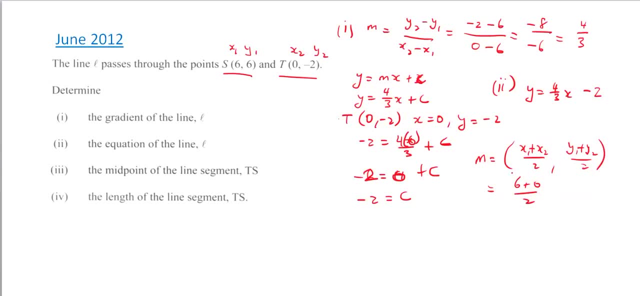 So we'll put 6 plus 0 over 2, comma And y1 plus y2 over 2.. So we're going to add the two x-coordinates, So we'll put 6 plus 0 over 2, comma. 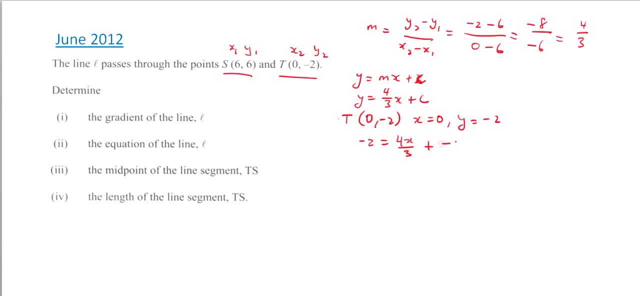 plus c, which is minus 2. sorry, what am i doing? plus c, right. so now what we should do is to get out of this tree at the bottom here, so we multiply everything by 3 and this will give me. minus six is equal to four. sorry, i made a mistake here. this is zero, right? so this will give. 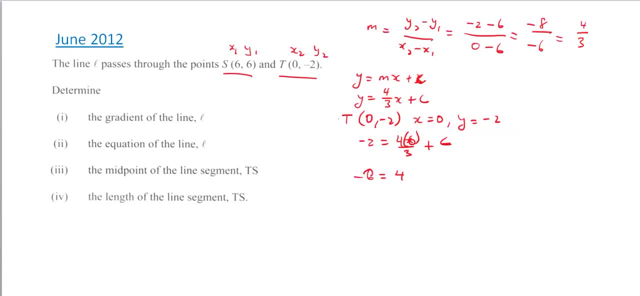 me sorry, i don't even need to do that. give this as minus two, and this will be zero plus c. sorry about that. so therefore, minus two is equal to c, right? so therefore the equation of the line will be: y is equal to four over three, x minus two. 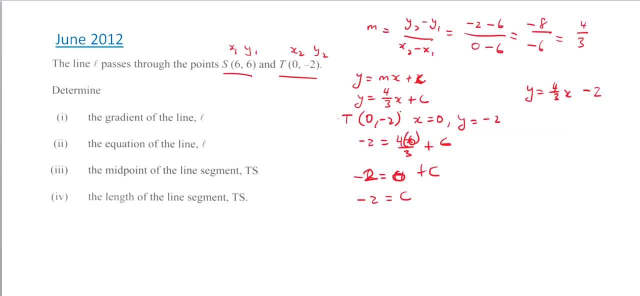 right. so this is the answer for the first part. this is the final answer for the second part. that is the equation of the line. now they want the midpoint of the line, segment t s. so let me work out midpoint. so midpoint m is equal to. you have to add x1 plus x2. 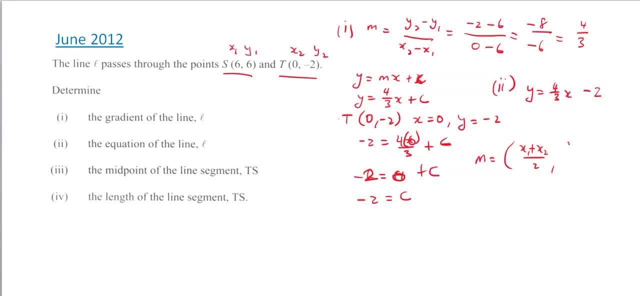 over two comma, y1 plus y2 over two. so we're going to add it to x coordinates. so we'll put six plus zero over two comma and six plus minus two over two, which will give me this will be six over three comma. six plus minus two is four over two, and six divided by three is two, and four divided by two is: 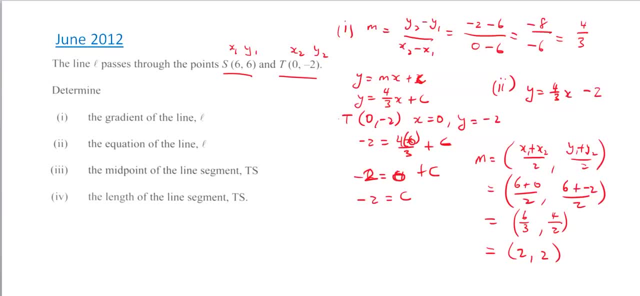 two. so the midpoint is two, two. okay, so that is the answer for third part and then the last part, part four: they want the length of the line segment ts. so first thing we do, we write down the formula for the line segment, which is x2 minus x1 squared plus y2 minus y1 squared, and we find the square. 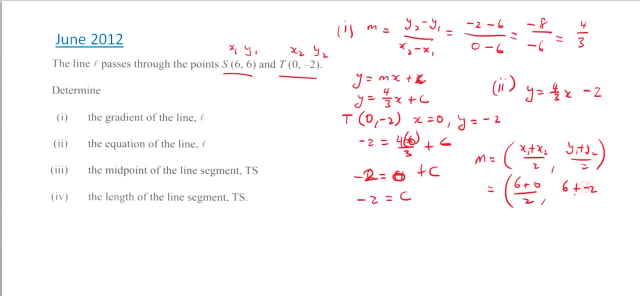 6 plus minus 2 over 2, which will give me this will be 6 over 3, comma: 6 plus minus 2 is 4 over 2.. And 6 divided by 3 is 2, and 4 divided by 2 is 2.. 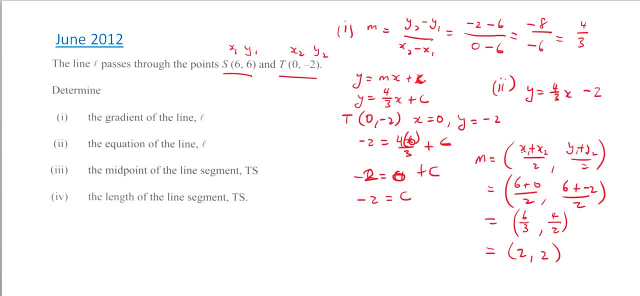 So the midpoint is 2, 2, OK, So that is the answer for the third part, And then the last part. So the midpoint is 2, 2.. And then the last part. part 4, you want the length of the line, segment ts. 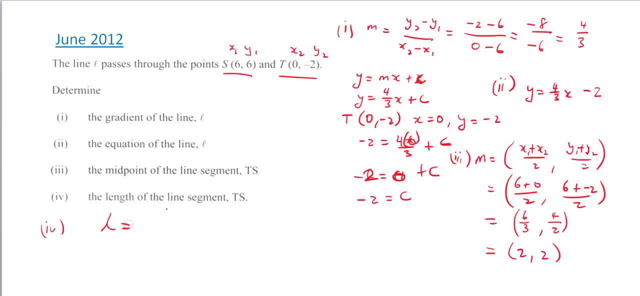 So, first thing we do, we write down the formula for the line segment, which is x2 minus x1 squared, plus y2 minus y1 squared, And we find the square root of all of this And, like I said, it's Pythagoras' theorem we're really using. 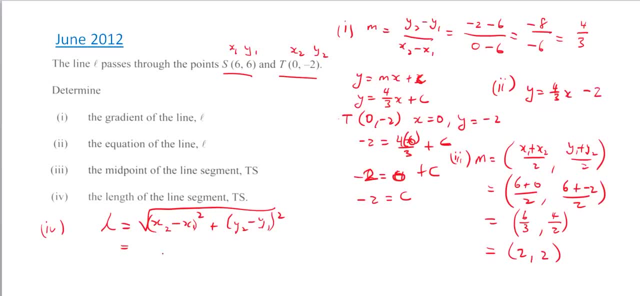 So we're going to use the square root And we're going to find the square root of all of this And, like I said, it's Pythagoras' theorem we're really using. So let's say so. it'll be 0 minus 6, right, because I'm substituting exactly what x1 and x2 is squared plus y2 minus y1,, which is minus 2 minus 6 squared. 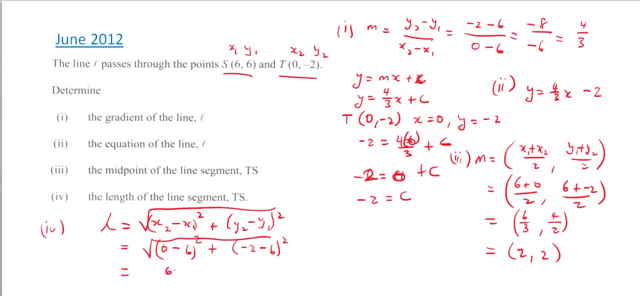 Find the square root of that. So this is really 6,. 0 minus 6 is minus 6,, right, so it's minus 6 squared plus minus 2 minus 6 is minus 8 squared. right, and this will give me 6x is a 36, plus 64,, and it'll be square root of that. 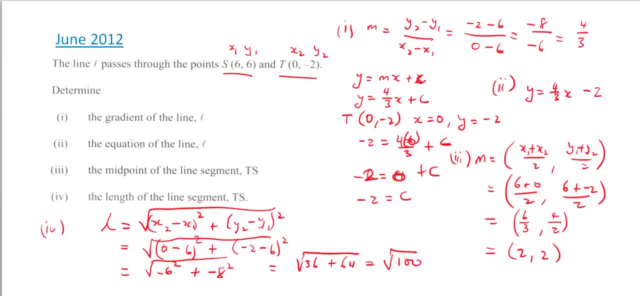 And this will be the square root of 100, which is equal to 10 units, right? So in this example, we applied all that we just learned: the gradient of a line, equation of a line, the midpoint of a line segment and the length of a line segment. okay,